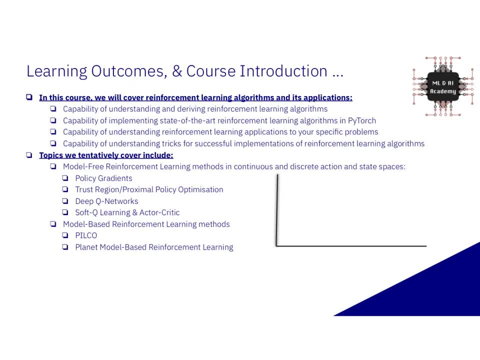 On a high level. we will cover two different types of algorithms from reinforcement learning. We will be describing model-free types of algorithms as well as model-based types of algorithms. In model-free algorithms, the agent that typically interacts with the environment does not assume any additional restrictions on the model of the environment that is under study. 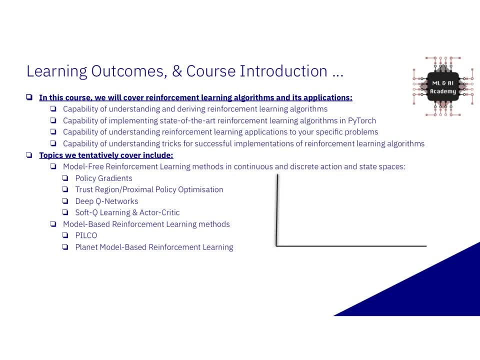 All it does is it interacts with that environment, gets some form of data, like traces or trajectories, from that environment, and then tries to learn an action selection rule in order to maximize its performance: The model-based setting. on the other hand, it tries to build a surrogate environment from the 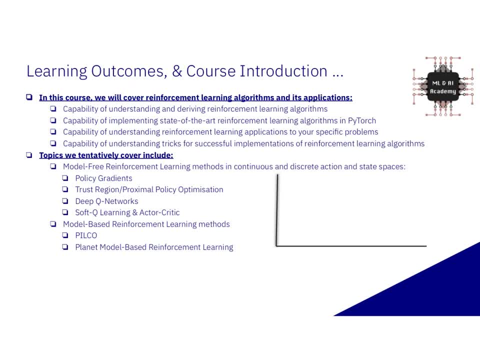 traces it had collected from the real-world environment. In that surrogate environment it tries to find the best action selection rule in order to maximize its performance. It thus updates the action selection rule of policy, Then it uses that policy to sample again from the real environment, and so forth. 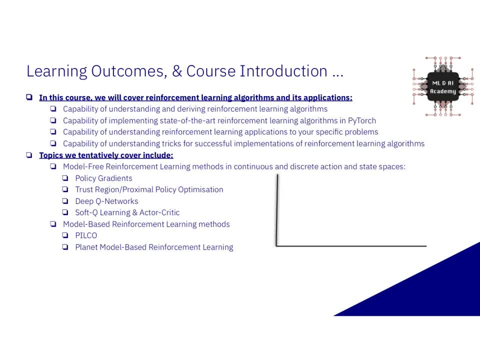 Clearly, doing model-based is much more sample efficient than doing model-free. So to illustrate this, if I am to plot a graph where on the x-axis I represent the number of episodes, so that's the number of traces or the number of times the agent interacted. 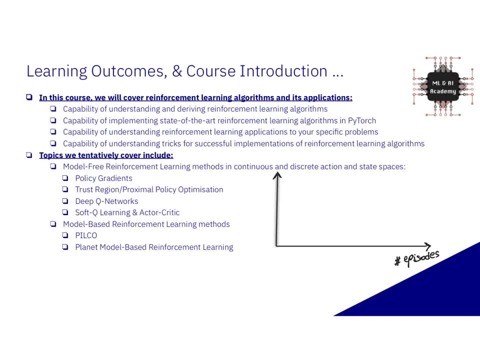 with the real-world environment- versus the reward. For now you can think about the reward as some form of a performance measure, so the higher the better. I try to plot this learning curve, which is reward versus episodes. You might see, for a model-free algorithm, a curve that looks like this: 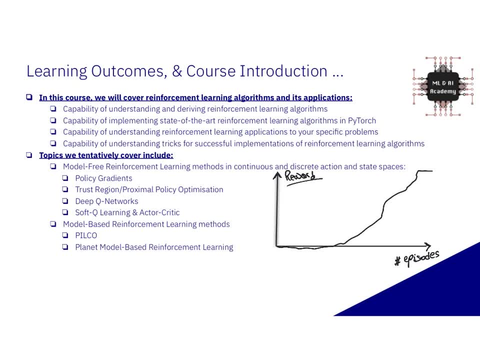 Of course, this is a made-up curve, but all I want you to see from this curve is: the more interactions we have with the environment. the more interactions we have with the environment, The more the reward is. So the higher the episodes, the higher the reward. 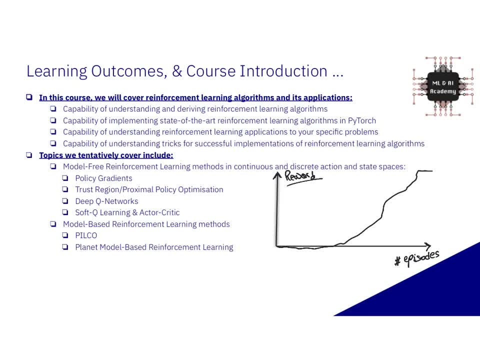 which means the agent is learning. Though successful current model-free, state-of-the-art, model-free reinforcement learning algorithms, they require millions, or maybe let's say hundreds of thousands of interactions to learn something useful. So this is all good, but when it comes, 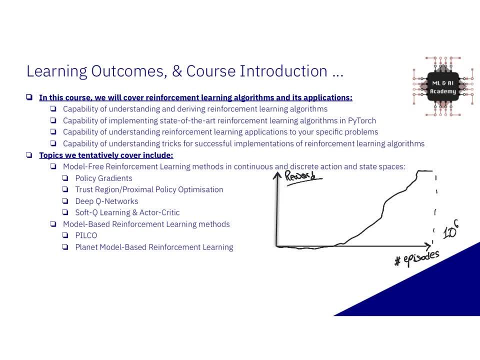 to real-world applications beyond Atari games. this is really really hard to apply, And that's where the model based counterpart comes into play, where, if I am to plot this learning curve for the model based algorithms, I would see a reward that looks like this where numbers here are in the tens: 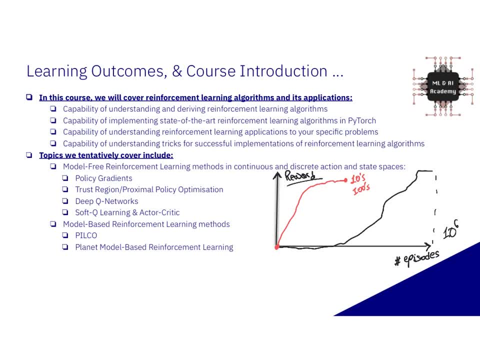 or hundreds of episodes. So all this is good and clearly, model based is more sample efficient than model-free. So why don't we use model-based all the time? Well, it turns out that model-based does not work really well yet in very high dimensional environments, such as, for instance, a 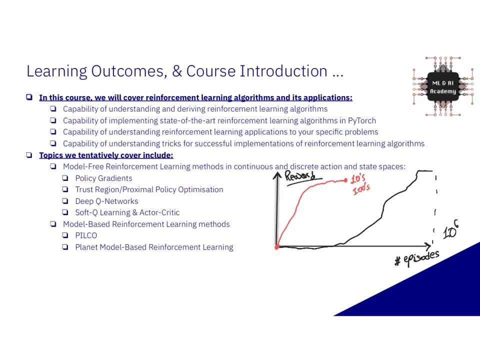 Atari games or any environment which has a state representation in the order of thousands, And that's why you have a trade-off to consider here, where you try to be as efficient as you can, depending on the dimensionality of your problem, And there are algorithms which reside in between. 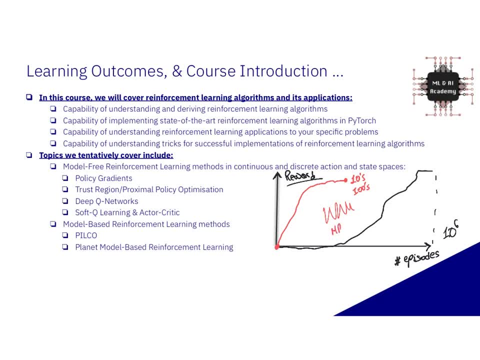 these two, which are like model-based, model-free- type of algorithms that try to get the best of both worlds. We will be describing these different algorithms and implementing some of them, together with the hope that you are able to understand when to apply the model-free setting. 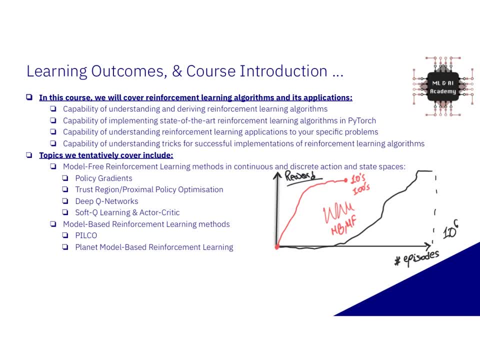 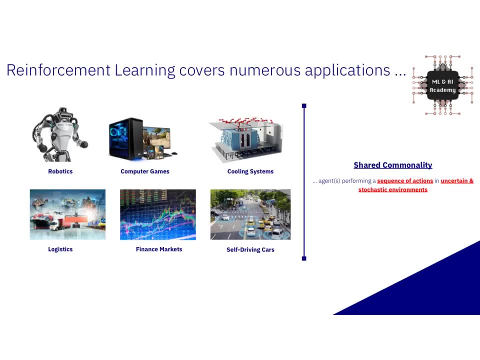 and when to apply the model-based setting. So at this stage, you might be wondering: why do you even attempt to learn reinforcement learning? Well, it turns out that reinforcement learning is a useful tool that can be applied to a wide range of possible applications: Applications involving robotics, computer games, cooling systems. 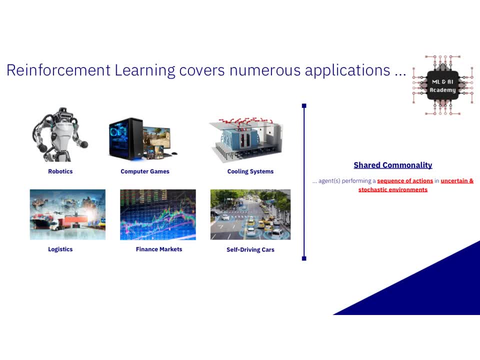 logistics, finance, self-driving cars, among others. In all these applications, you always have an agent and that agent is trying to perform a sequence of actions in the environment which is uncertain and stochastic. So what does that mean? So imagine you have the car in a self-driving car scenario and that car has to go from a place. 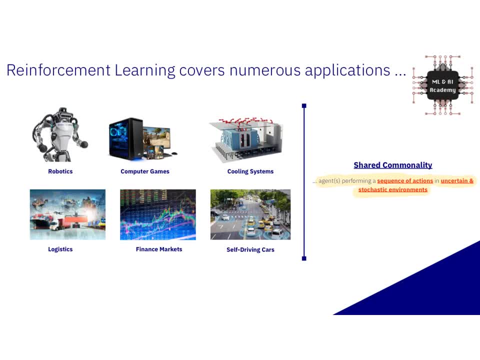 to another. So at every state on the road the car takes an action That transitions it to a successor state. However, this transition itself is not deterministic, in the sense that if the car had applied the same action again in that specific state, it might end up in a slightly 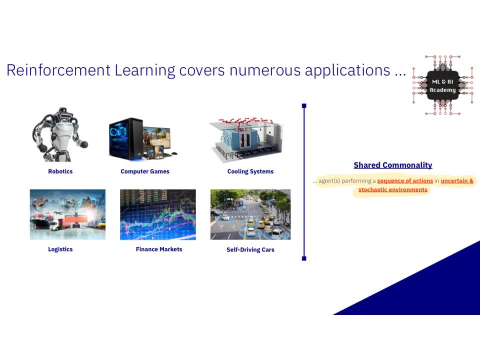 different state. So if the car had applied the same action again in that specific state, it might end up in a slightly different success. The reason for that can be, for example, random sensors or noisy sensors. The environment itself might be stochastic, So, for example, a pedestrian suddenly decided to pop up and so forth. And now 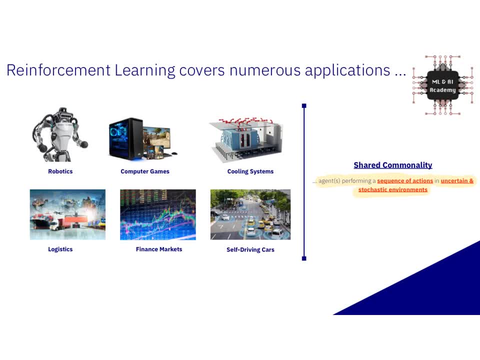 the goal of the car is to take a sequence of actions such that it maximizes some notion of performance. So, for example, in the car it shouldn't crash, it should have a safe driving maneuver, etc. etc. So in general, a lot of problems can be described as instances of reinforcement learning, where we 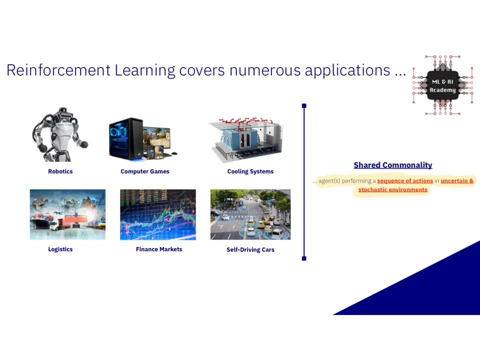 have an agent that is performing a sequence of actions in an environment which is uncertain and stochastic, with the goal of maximizing a notion of return. It is important to note that there's a temporal nature to this problem, So we're not only interested in one-step action. 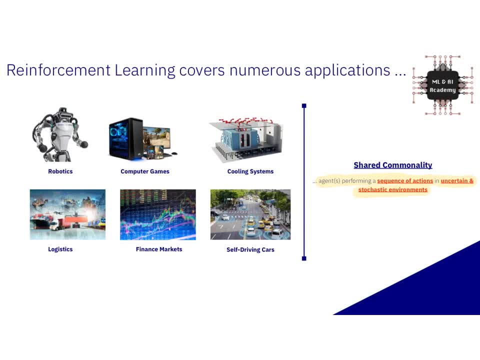 application, but we're also interested in one-step action application. So we're not only interested in one-step action application, but we're also interested in one-step action application, But we're interested in a sequence of action applications. And the reason of that? because there's a trade-off. 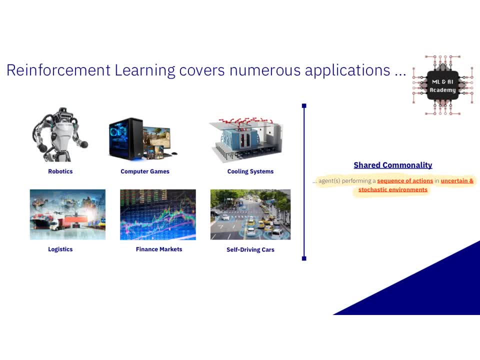 between immediate action and future action applications. And that's what makes the problem a little bit more difficult, Because now you cannot just be greedy in the sense of taking the best action at this time step, because it might hurt you after 10 time steps. So this is the 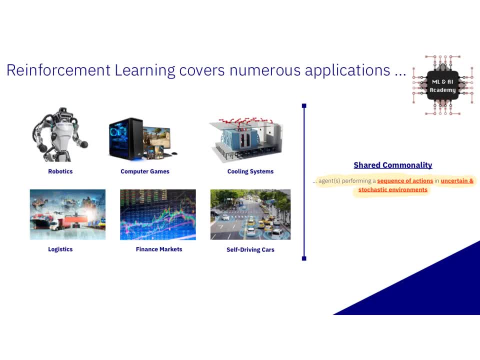 trade-off that reinforces the problem And that's why we're interested in a sequence of action, applications And, as a general rule, that reinforcement learning has to consider a QA on what done not to attain dis ubiquitously. That's a good faction, because the biggest sambol 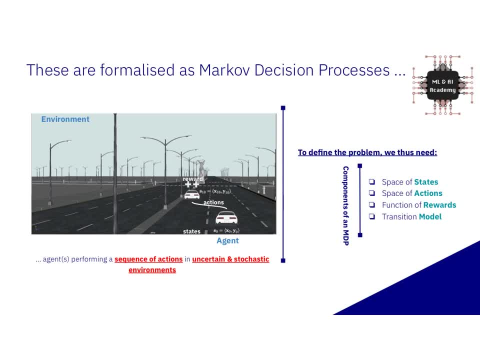 we have in order to obtain resolute action and have the basic understanding that reinforcement learning has also to consider in order to attain a successful action selection rule Right. So by now we have understood that in reinforcement learning we have an agent that is performing, as we agreed, a sequence of actions in an environment that is typically 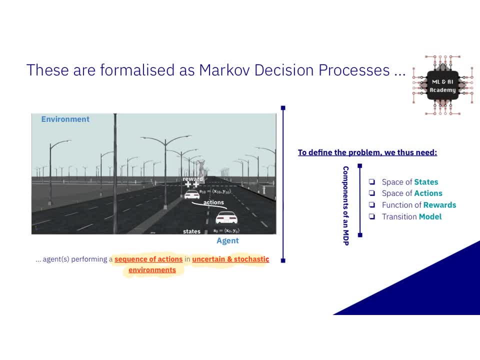 so to depict this idea, I'm just giving an example here where I have a car which is our agent in an environment which is like the road and let's say the car's goal is maybe to navigate the road, you know, go from a place to another. 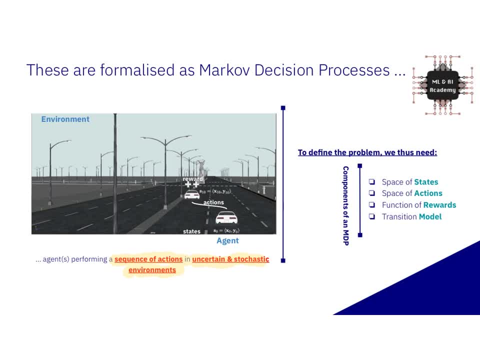 comfortably, safely and without crashing. so here we need a couple of things to be able to define this problem. the first thing we need is we need a set of states. so, for example, the car starts here and applies some sort of action so that after 10 steps it reaches there. so we're gonna use here, in this example, the X and Y. 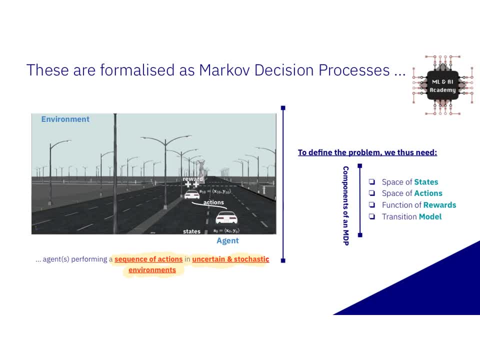 position of the car as the state description of that car in this environment actions can correspond to, maybe, you know, like go left, go right, or throttle a break and so forth, and these actions are gonna dictate how the car moves from a place to another in this environment. so the way this car moves in this 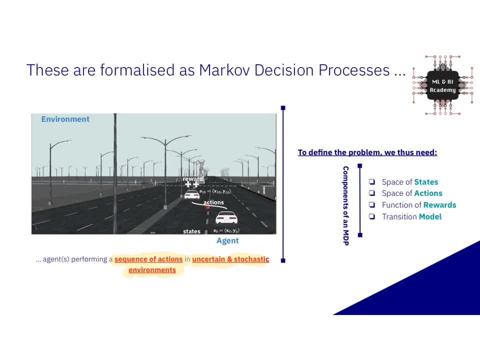 environment dependent on the state it was in, and then action it had applied takes the car to a new state according to a model of the environment which we call a transition model. In addition to that, we need some form of performance quantifier, which is what is denoted here by the reward. So the reward is going to 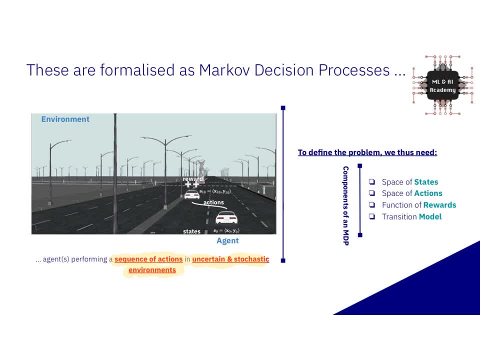 tell the car: you did well, so you get like a plus plus reward. So, for example, if the car didn't crash, then it gets a plus plus reward. But if the car, for instance, does some unsafe move, we can give it a negative number, and then the goal is to reinforce the positive numbers or the good things. 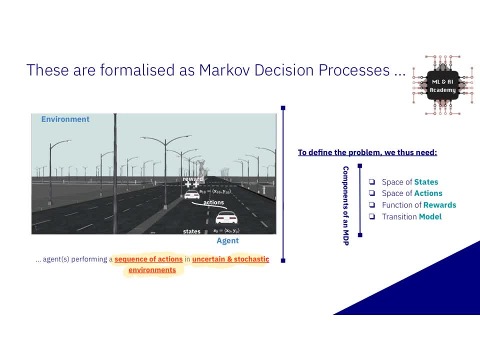 that happened in these traces or trajectories the car has executed in the environment. So, in short, to define the problem we need four components. The first component is a set of states or the space-time, So the first component is the space-time. So the first component is the space-time. 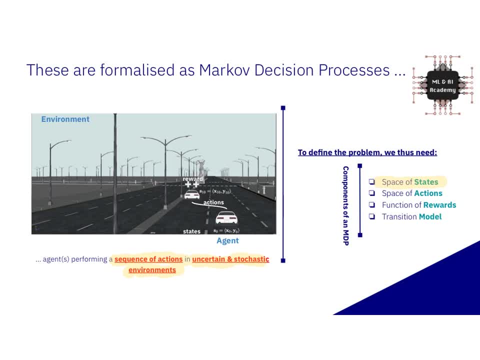 of states. So these are, for example, the xy position of the car. We need the space of actions, So that's like the action set that we are going to allow the car to execute. We need the reward function, which is going to tell me how good the car is performing, And we need the transition. 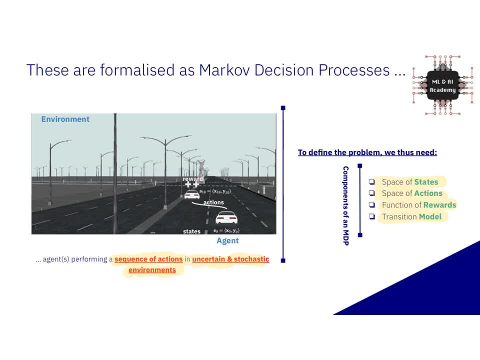 model, And that transition model is some form of a stochastic equation that dictates the change of the car's performance. So we need the transition model, which is some form of a stochastic equation that dictates the change of the car's state, conditioned on a previous state and an action. 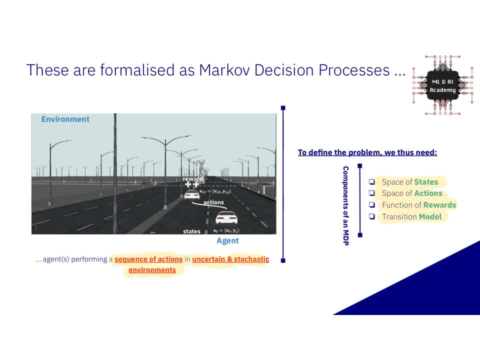 that has been executed. There are different types of these states, actions, rewards and transition models that we consider in reinforcement learning. So, for example, the set of states can be continuous, as is the case in this car experiment. So here we say that the state of the car is, for example, 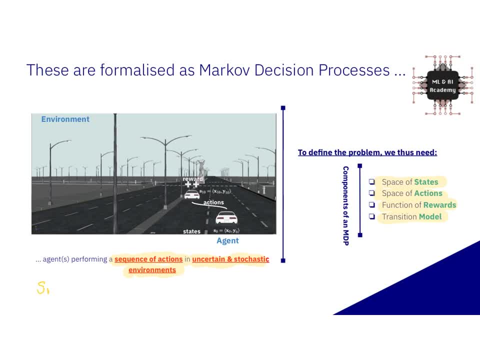 in R2.. So we say that the car state of the car belongs to R2, which means simply that the car's state is a two-dimensional vector, each being continuous. So in other words, when I write a notion that looks like this, I really mean that this is a vector of two constants. 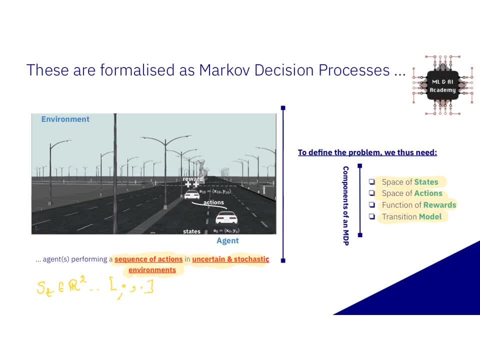 and we say that the car itself is a two-dimensional vector and that each component is a vector number. So here we have two components, And each component here is a real number. States, however, can also be discrete, not only continuous. So if you consider a grid-world, 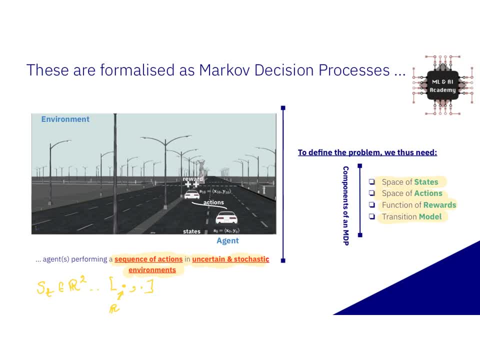 experiment. here the agent can go from a cell to another cell, dependent on the actions it had applied. And there we have a set of discrete states that the agent can belong to And that is also possible to define in reinforcement learning. Similarly, the action space. 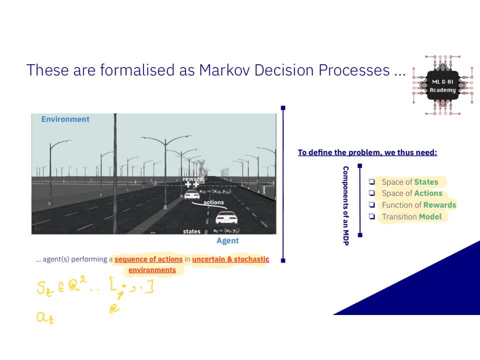 So the action space AT here, for example, is: let's say, maybe we're going to have a steering, braking and heading angle. let's say So, for instance, the action space is R3, which means again that the action is a three-component vector, each being a real number. 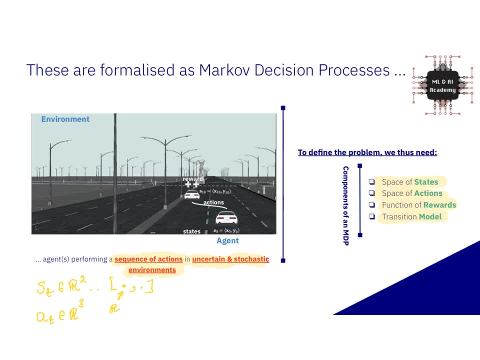 The reward is typically a function that takes as an input a state and an action and it gives me a real number. So we typically write that, as you know, you have a reward, function R that is going to take from you some state at time- TST. 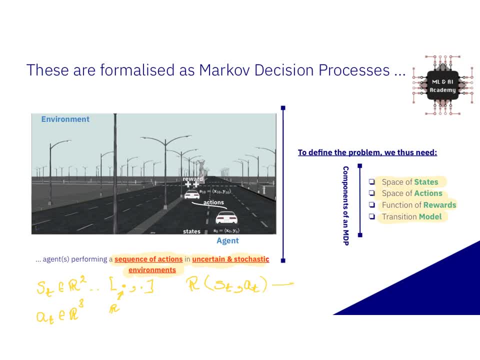 And that's going to be a reward. function R, Some action at time, TAT, and that is going to be some real value which is going to denote if this state and action that has been executed by the agent is a good or a bad action to apply in that state. 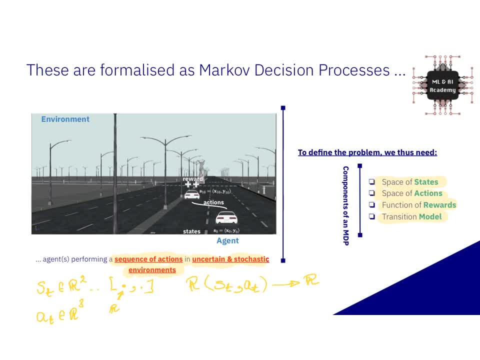 So if you get a positive number that's good, If you get a negative number that's bad. So mathematically, what we can do is we can write this reward R to be A mapping or a function really from the state space across the action space to the set of real numbers. 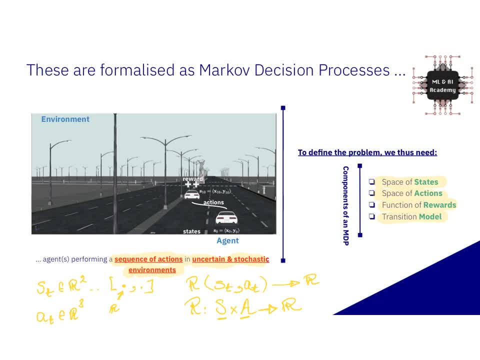 So this is a state, this is an action space, and that is mapped to the real numbers, and this is what the reward function is supposed to be doing. When it comes to the transition model, this is a stochastic transition model, which 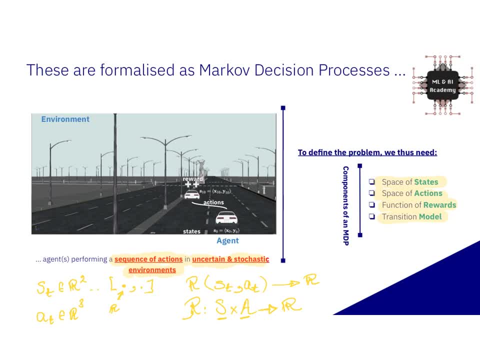 And the goal of this transition? The goal of this transition model is to dictate how the state evolves over time, depending on the actions applied. So if it was deterministic, your transition model- let's call it F, for example, your transition model F- would be some function that will give me, for example, set value of the state as T. 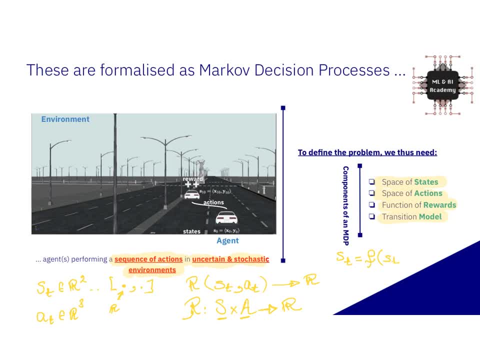 So that's the F, the transition model, as a function of the previous state And the previous action that has been applied. As we said, however, this transition model is going to be stochastic And that's why it's not going to look like a function F like this, but it has to look like a probability density. 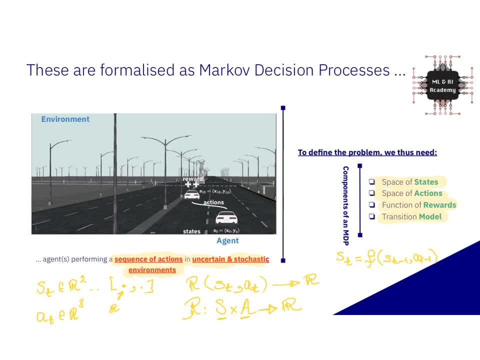 typically a conditional probability density, which we will write as ST conditioned on ST minus 1 and AT minus 1.. We will dive into This in the next slide, But all I want you to get is to define this problem of reinforcement learning. 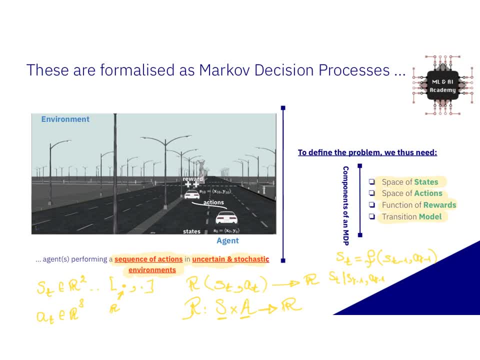 We need a set of states or a space of states which is, as we said here, can be like R2 in this example. We need a set of actions, like we described here. We need a reward function and we need a transition model, which is typically a conditional transition model. 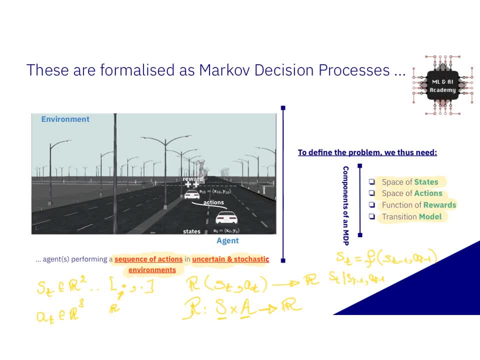 So for you to fully understand These, you need a primer on probability and densities. So please check out the other lectures we have on our channel where my colleague describes this notion of probability densities much clearer. What we're going to do next in these slides is going to give an example building on top of that. 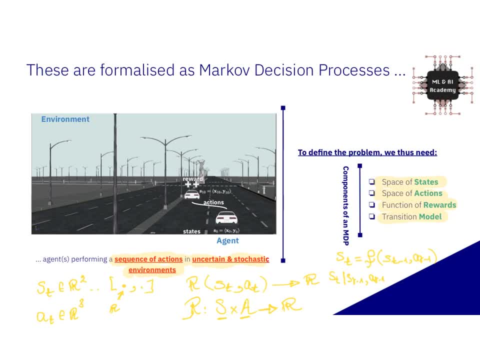 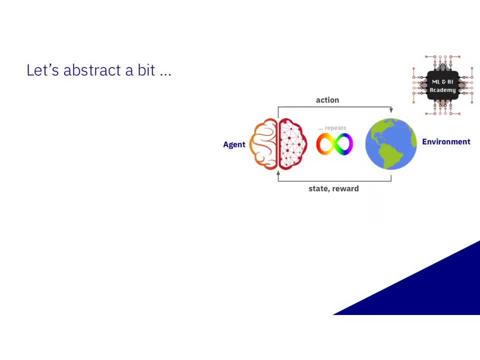 but please do check that lecture for you to fully comprehend the mathematics behind these transition models. Right, so what we would like to do now is we would like to understand these notions that we derived before much better by maybe giving some examples, but let's do that at a more abstract level. 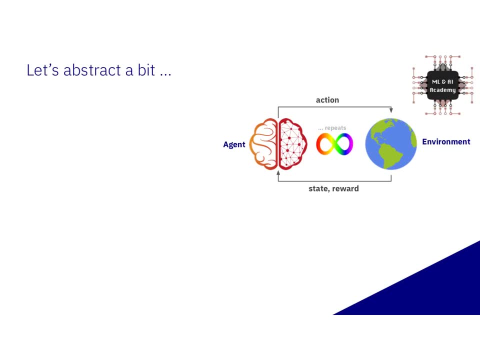 So, rather than having the car agent interacting on a road environment, let us just say that we have an agent and that agent is talking to some sort of an environment. The way it interacts with that environment is by applying some actions on that environment. 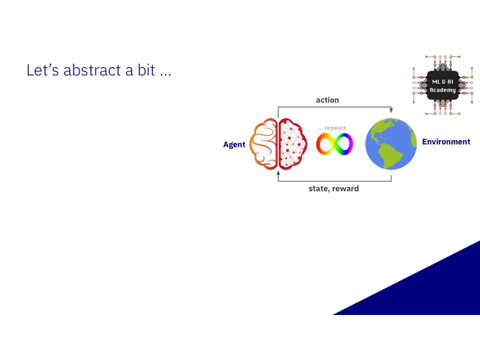 The environment then responds by a state and a reward. Now this process repeats, right? So in this new state, the agent then takes some other action And, as you remember, we had this notion of sequential actions. so now, given a new state, 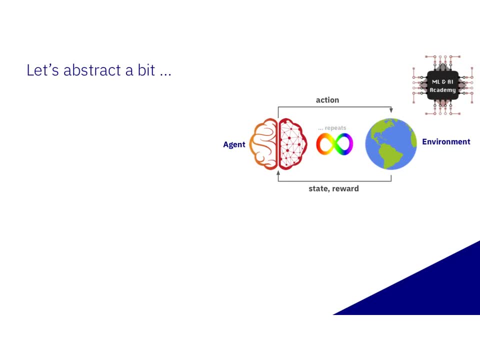 the agent takes another action, the environment responds by a new state and a reward, and so forth. So, as we said before, we're going to need a couple of components to be able to define this problem. So the first thing we need is we said we need a state space. right, So a state space. 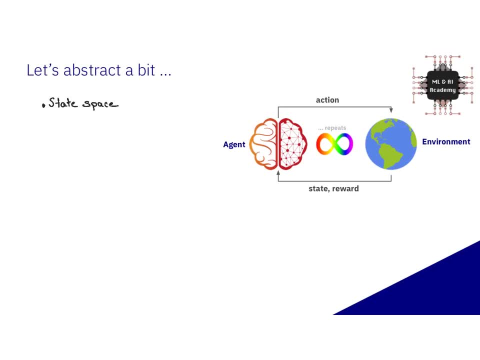 where each state belongs to, And we're going to assume for now that the state space S right is some continuous state space. So it is belonging, so it's a subset of a d-dimensional space. What this notation means? it means that every vector, when we say ST, belongs to this state space S. 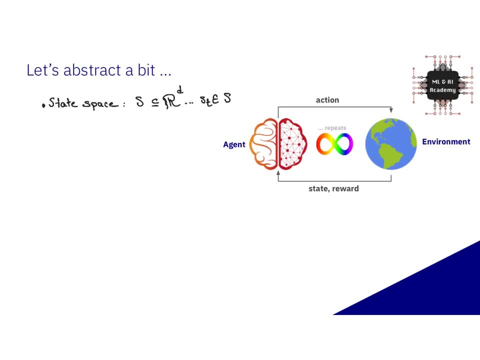 we simply mean that this ST is a d-dimensional real vector where each component belongs to this state space S. So we simply mean that this ST is a d-dimensional real vector where each component belongs to this state space S. So we simply mean that this ST is a d-dimensional real vector where each component belongs to this state space S. 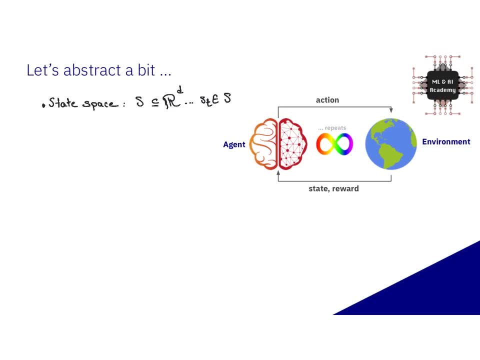 So we simply mean that this ST is a d-dimensional real vector where each component belongs to this state space S And it has size t and that real number can be just from minus infinity to plus infinity. We also said that we need an action space, as we described before. 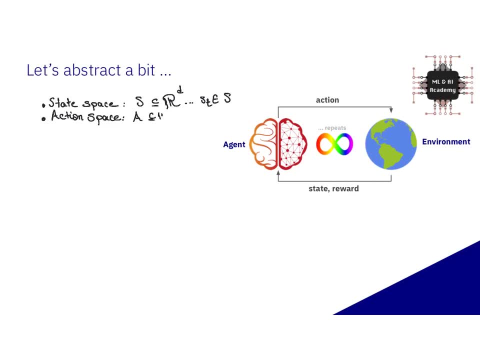 So our action space A, that's another d-2 dimensional space, And when I say that AT belongs to A, I mean that AT is a d-2. dimensional vector. each component in that d2 dimensional vector is a real number that can be. 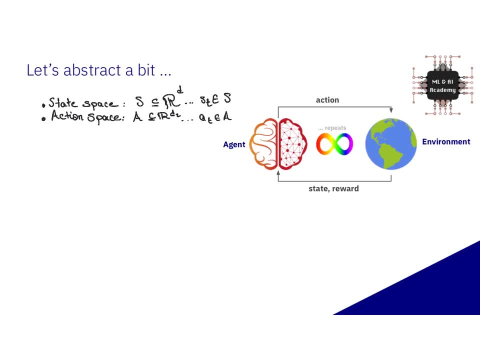 between minus infinity and plus infinity. So that's all good, but now we need a couple of additional components, as we described before. So we need it. for example, as you remember, the reword function, And that's a function that is going to simply map, so r we're going to call. 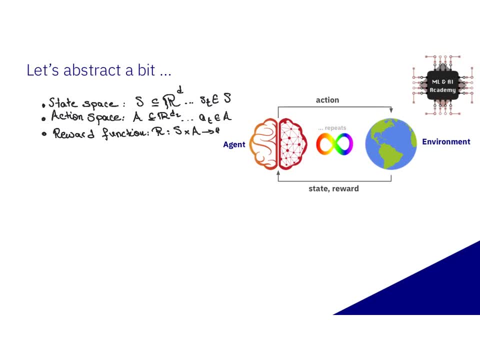 it that's going to simply map from s cross a to the real numbers. So you can think about r as some form of like a box, right? So this is a box. It will take some st which is in this space s. 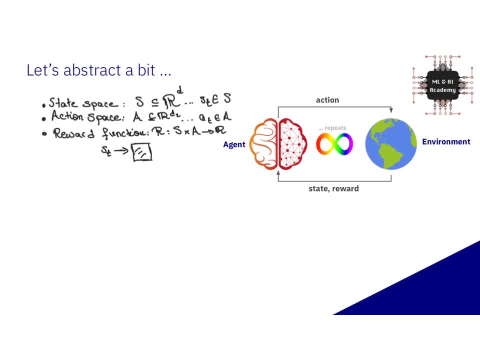 right. So this st is in this space s And it's going to also take some action at right, And that action at is in this space And on the output it will produce some real number right. So that is going to be just some. 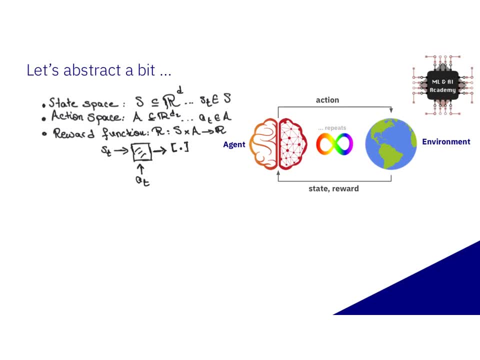 real number that somehow quantifies the performance of our agent. Now, please notice that the reword function can also be stochastic in its own right, but we're not going to discuss that just yet. We're going to assume that the reword function is something that is given. 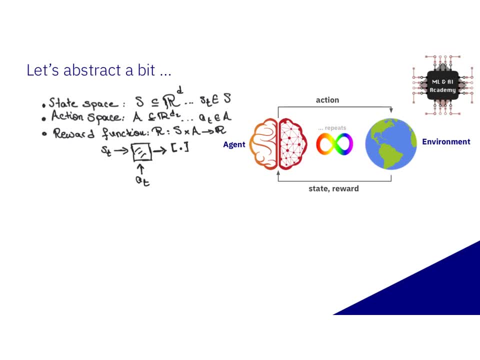 All right, And that reword function is just a map or a function that takes a state st and action at and gives me a real number. Now what makes reinforcement learning hard is that typically this reword function is not known to the agent in a sense that the agent can exploit the reword. 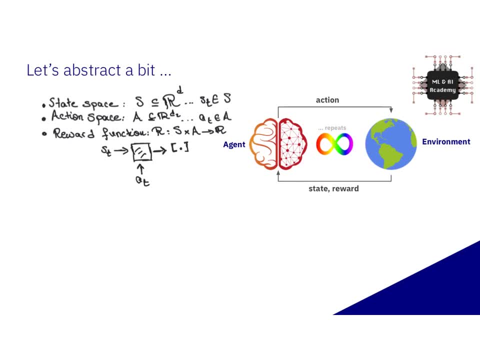 function to learn something useful. The only thing the agent has is just set of numbers of like plus one or minus one or zeros, and they are typically very sparse as well. So you get a reword function which is always zero and then suddenly plus one, And then from that the agent 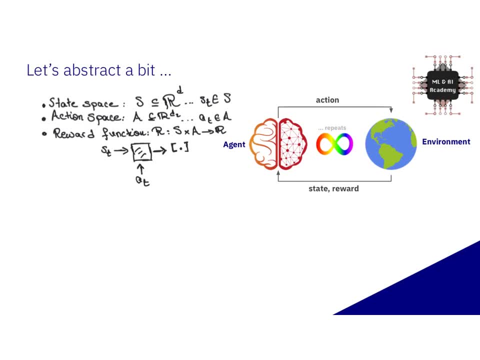 has to learn how to apply a set of actions correctly in order to maximize that type of total reword that it would get. Another component we mentioned is the transition model, and that's what we're going to dig into a little bit deeper now. 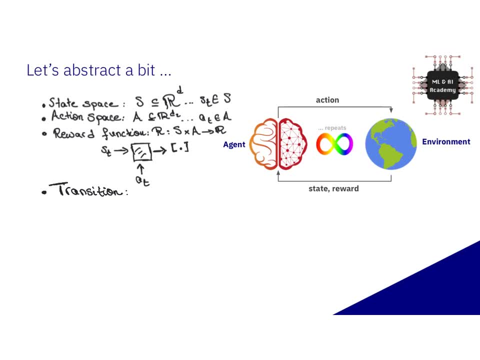 The transition model. we said it was a stochastic map, right? A stochastic map that takes from me some state and an action. It gives me some distribution or density over successor states. So the way we're going to write this, as we said, is we're going to say that: 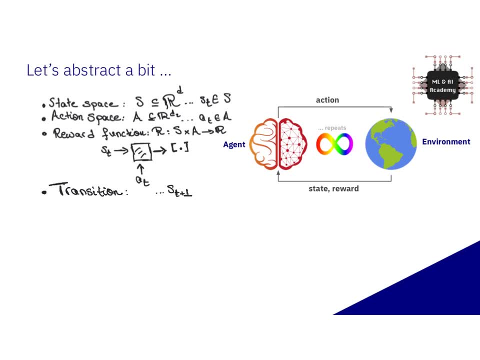 my state at time, step t plus one is conditioned on the state at time t and the action at time t. and now that means that, given some state st applying an action at, there is some form of a conditional density over st plus one, which means that st plus one does not take the same value every. 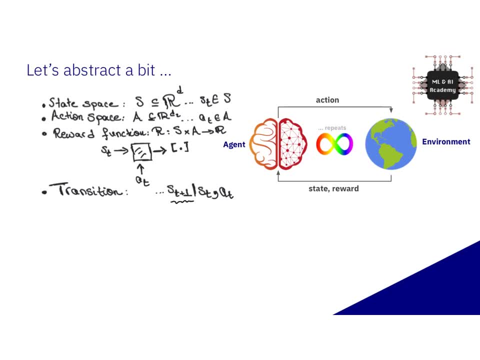 time we apply the same st and the same at. So this map is kind of a stochastic map To better understand this right. like the simplest form of this map, we can say that, all right, we're going to have st plus one right, as we said before, to be some function of st and at right. 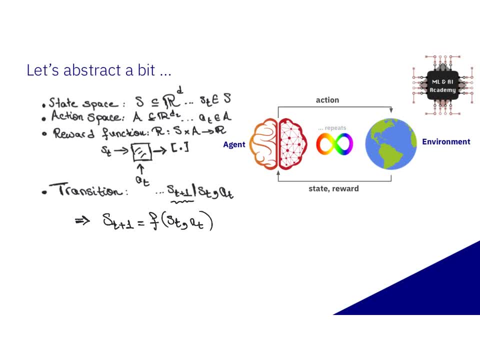 So that is like the dynamics you know like. it's just like, for example, in a Mario game, awkward function which is hard to determine, but it's like a function where you have Mario here, then it says jump, then Mario jumps, so the next frame is: 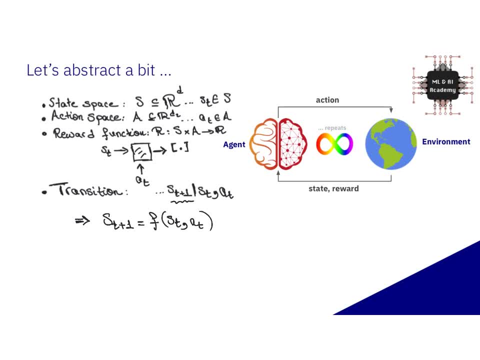 Mario jumping. so that's st plus one, and the function is what maps this Mario jump to the new frame of jumping. but in order to make this stochastic, we're gonna need to add some form of randomness into this equation. a very simple way to do this and that's not typically very successful. but like just 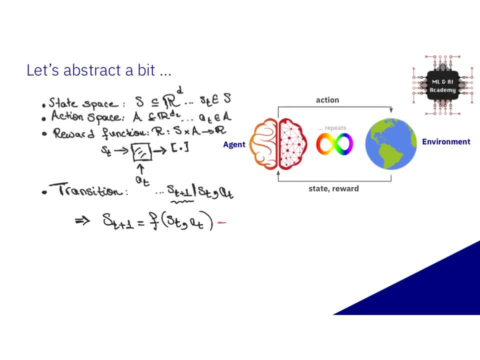 to understand. a very, very, very simple way to do this is we're gonna say: okay, I'm gonna add some noise epsilon to this equation, right? so what I'm saying is that the noise itself is random, so that is a like a random number, for example in: 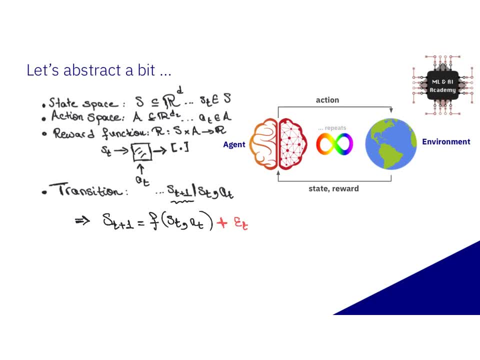 in Python you can write that as NP, dot, random, dot, normal or something, so that's like a random number. so that means that this guy- because this is a random number, every time this guy can take different values depending on the samples you get from that distribution. right? so you know, we have, you have some distribution, so we 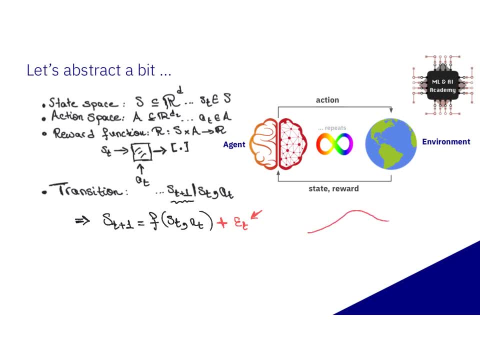 have like, let's say, for now it's a, it's some sort of a Gaussian distribution, let's say: right, and then every time you ask a sample right from that distribution you can get a different value for this epsilon tee, right. so that means that that the idea here is that this, because it can take 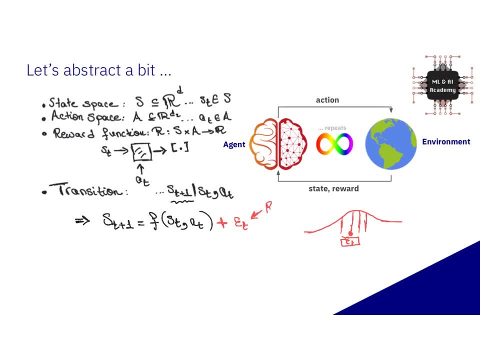 different values. it's in fact a random variable. so now we add it to this deterministic equation. some form of a random variable noise coming from some distribution. The way we write that this guy is coming from some distribution, which is denoted in this notation, which says that guy is sampled from some distribution, right so? which means that 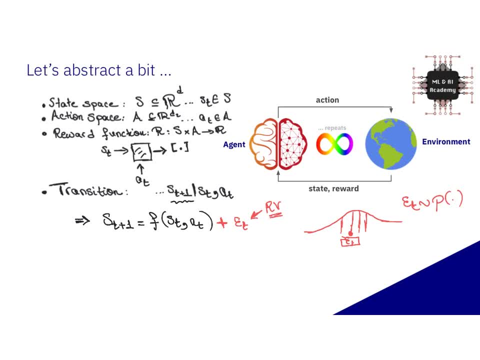 epsilon t is a random variable. it has some density or distribution and every time you instantiate epsilon t, you observe a value of epsilon t. what happens is you sample from this distribution p, But now notice that, because this is a random variable, right, that makes. 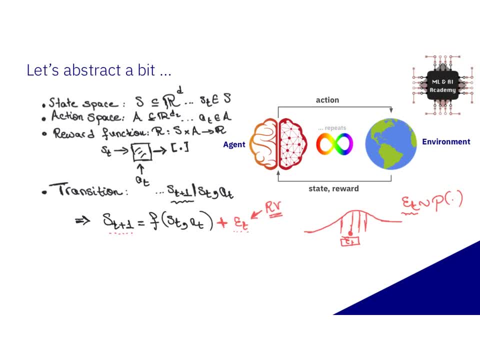 this also a random variable, which means now St plus one is not just one value that you will observe, Even if you had applied the same St and At to this function f right. so even if the function f took a random variable, if you just apply the same value to f right, you can get a. 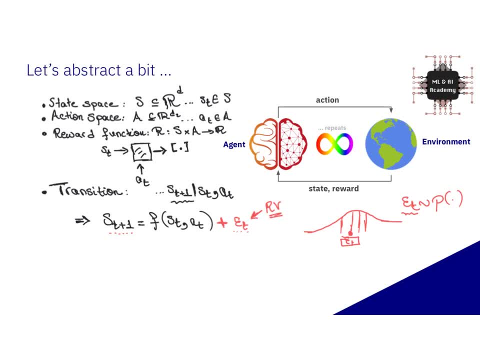 random variable. So even if the function f took a random variable right, even if you had applied the same st and at, due to the possibility of observing in the same st and at different epsilon t values, because it's a random variable, then st plus one is also a random variable. 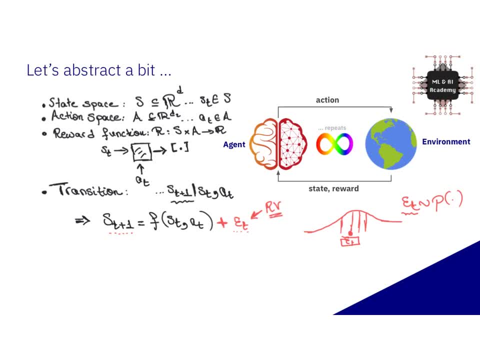 So this makes this transition stochastic right, which in turn means that every time I observe st and at, I can observe a different value for epsilon t, which means I can observe a different st plus one. So why would anybody care for this? I mean, there are a lot of reasons. 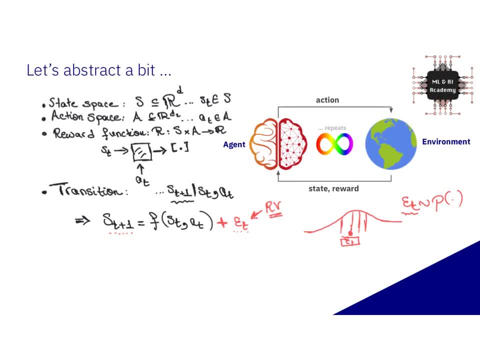 but it turns out that most real-world problems are stochastic of this nature. So, for example, if you are considering a car and now you have some sensors that measure the position of the car, these sensors are typically noisy, so you have to consider them stochastic, and so forth, But now we know that we have a state space right, which is just 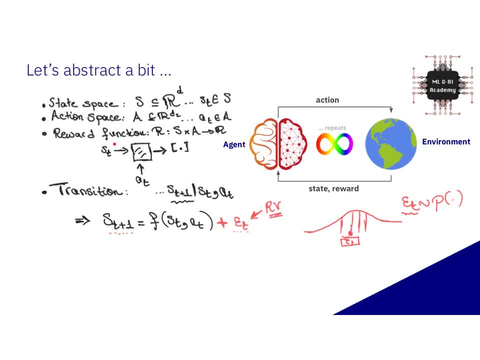 some vector, an action space, some other vector, a real-world function- that takes the state and the action and gives me a transition and gives me- sorry, a real value. And we have a transition which is typically stochastic. so we write it in this way: We say that st plus one is conditioned. 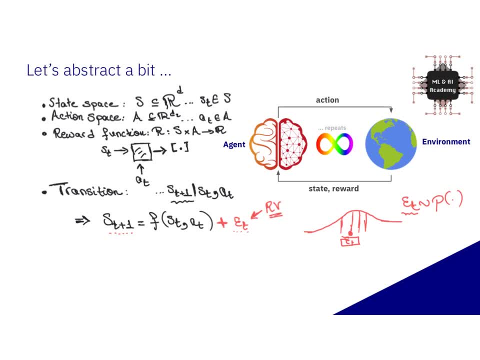 on st and at, and what we really mean by that is that this is sampled from some probability density that's called p-transition or something, and that is a conditional form of density. So maybe I can illustrate this a little bit better by assuming, just like let's go through a 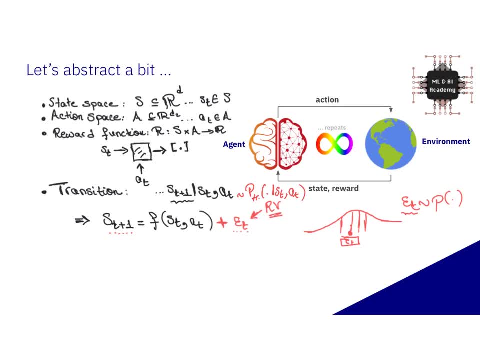 simple derivation of like some linear equation. So we're going to say that: okay, imagine that my st plus one. so my next state, let's say, for now it is a one-dimensional vector, so that means that d is equal to one in this scenario, And 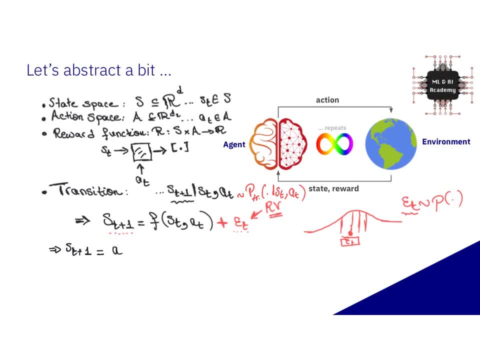 let's say that, well, you know what this is going to be like, some equation which is ast plus but, and plus some noise, as we said there right? So the idea now is that we're saying that st plus one is a 1b vector. 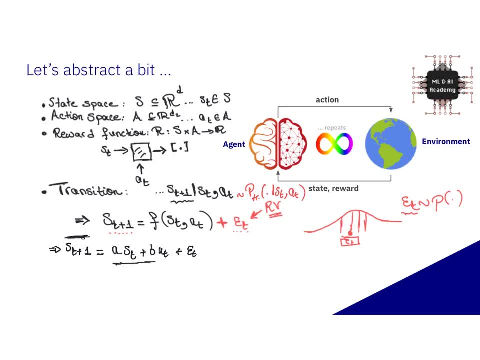 that results from a linear transition where you have ast plus, but sorry, ut should be at. so that's just the action and we're going to add some noise to this process, right? So this is going to add some epsilon t. 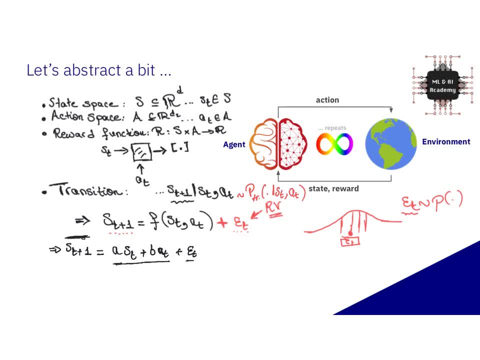 some noise to this process. Let's further assume that this noise, epsilon t, is Gaussian noise, which has a mean zero and a variant sigma squared. So when I write an equation like this, I simply mean by it the bell curve, and that bell curve has a mean, which is the expectation of epsilon. 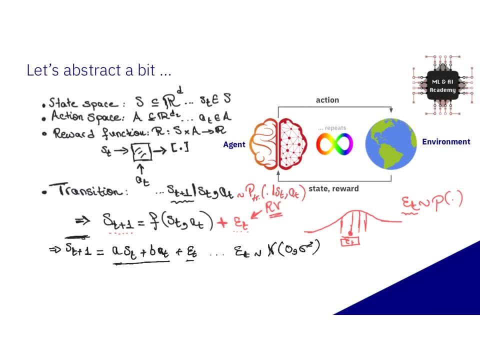 and a variance, which is the variance of epsilon t. Now, with this you can derive the fact that st plus one given st and at is also going to be sampled from another Gaussian. okay, The mean of that Gaussian is going to be AST plus BAT. 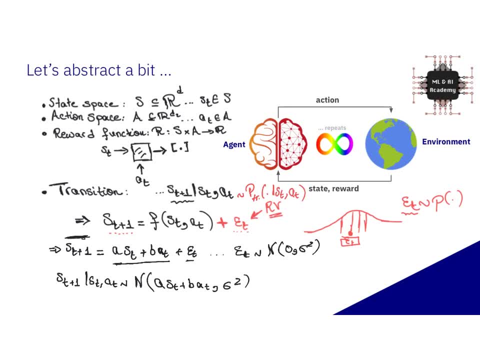 and the noise is going to be sigma squared. Don't really worry where this came from. We'll derive this later in the lecture, But now this is interesting to understand. So what this is saying right, is that if your noise was Gaussian, okay. 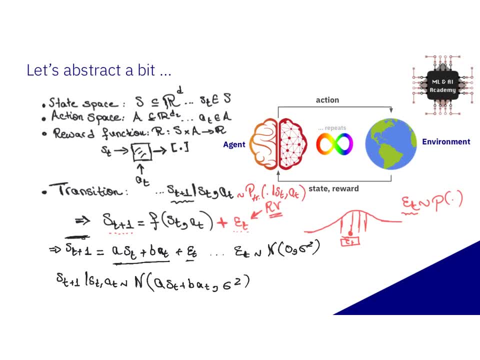 then your successor state ST plus 1, conditioned on ST and AT, will also be a Gaussian and it has a mean around AST plus BAT and it has some sigma squared variance. So that means that anytime you are at the state ST and you apply an action AT, 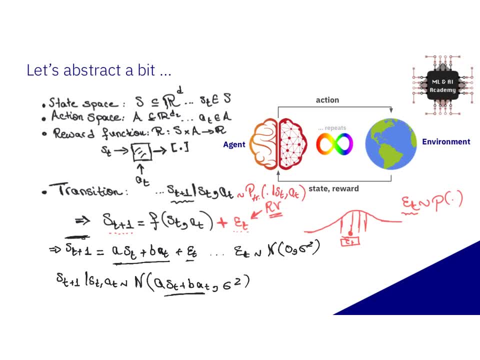 your successor state. your successor state can be as Gaussian distributed, with that mean and that variance. In other words, if you have a block, that is like your transition model, so you can take here ST and you can take here AT, and that gives you ST plus 1.. 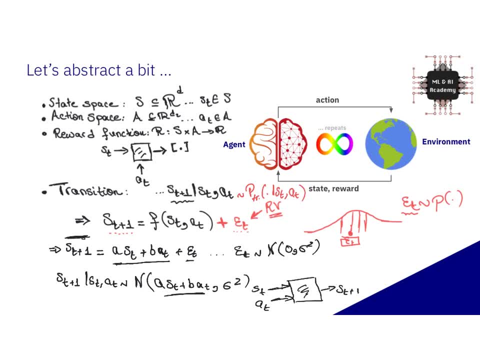 If you are to apply this ST and AT multiple, multiple times, you will trace on the output some form of a Gaussian with a mean. So you will trace on the output some form of a Gaussian that maybe looks like this, And the mean of that Gaussian is going to be AST plus BAT. 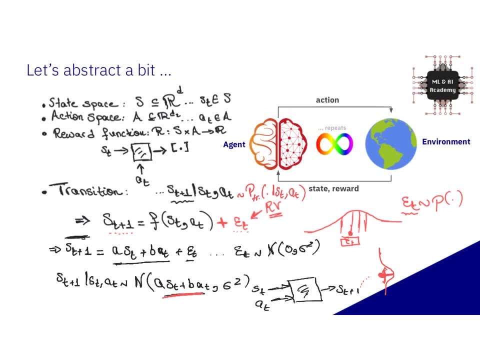 and the variance of that Gaussian is going to be the same as the noise variance, which means that with time, as you observe this over and over and over again, then the distribution of this guy is going to be the Gaussian, with the mean being the kind of deterministic part. 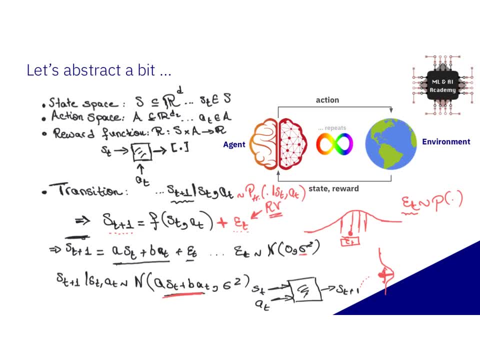 of this equation and there's some variance: sigma squared. Now, what makes RL also hard is that the agent does not have access to this function F, because if it had, it can in fact exploit this function F right. And then, based on that, 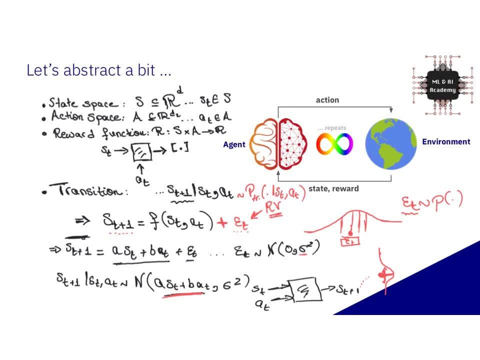 you can try to determine a very good behaving action selection rule and then, based on that, you can try to determine a very good behaving action selection rule and then, based on that, you can try to determine a very good behaving action selection rule. 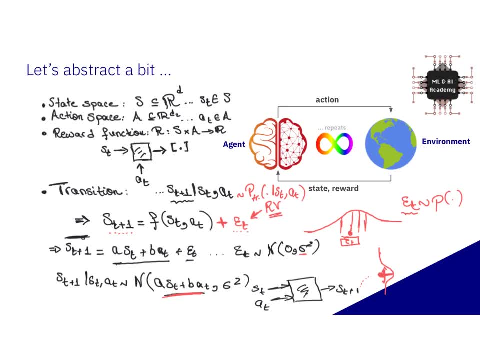 and then, based on that, you can try to determine a very good behaving action selection rule in order to have good action selections to maximize your performance. If you think about optimal control, optimal control is very, very related to this setting of reinforcement learning. 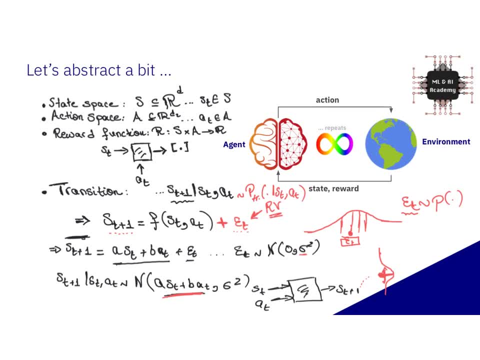 but in optimal control you typically assume that you know your transition model F. Here we're going to assume that we have no clue about the transition model nor the cost function. That being said, there are forms of optimal control that also don't consider the transition model to be known. 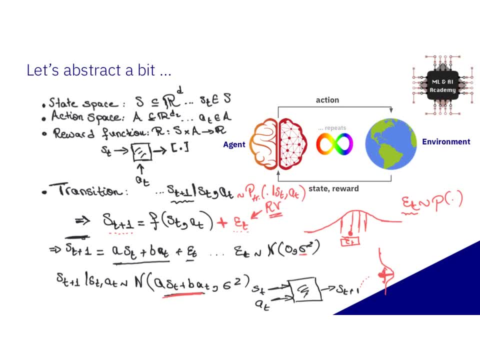 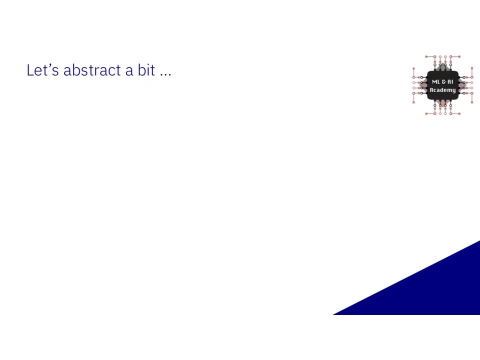 but we're not going to assume that Let's go ahead and dive into these just yet. Yes, right, so far we have understood what is an MDP, We understood what is a rework function, What is a transition model, And we understood that the generic goal is to find: 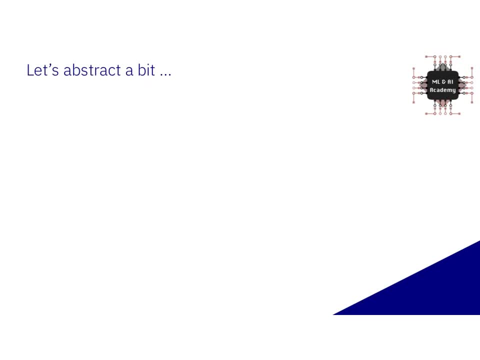 some sort of a policy or an action selection rule that dictates a good behavior. so the remaining part that we need to describe before going forward is this action selection rule. so remember that at every time step t right, our agent is executing an action at right. so 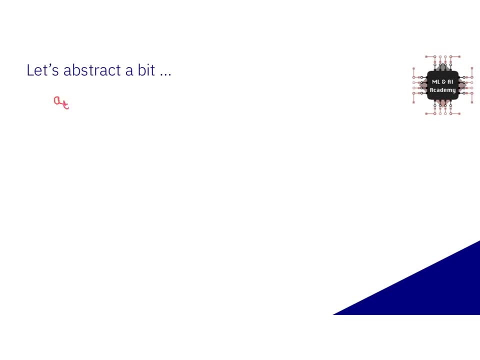 we're going to have some action at at every time, time step t executed by this agent. what we're going to say is we're going to say that that action a, that action at right, for it to be informative, it's going to be some function of a state st. 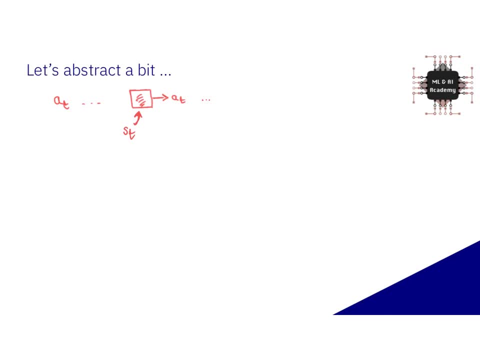 so, in other words, you give me a state, then there's some function or some map, really, because at can be d-dimensional, that will give me 80. Now this function itself, right, can be also parametrized. So, for example, you can have a neural network here, and we will dive into this. 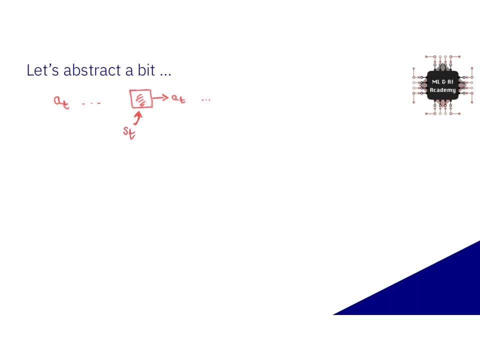 in a second, But for now we need to have some function that will pick the actions, and we're going to look for the best sort of function that picks the best actions to maximize performance. That's kind of the goal right. So we need the best. We're going to call this function a. 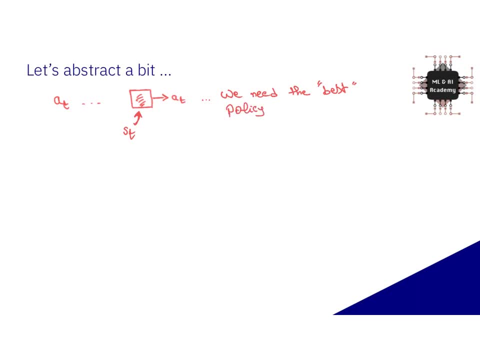 policy right. So we're going to need the best policy, which is like the action selection rule: We need the best policy. That's what we're going to do, So we're going to try to find the best policy. So here there are some notions to understand. still, What do we mean by best? 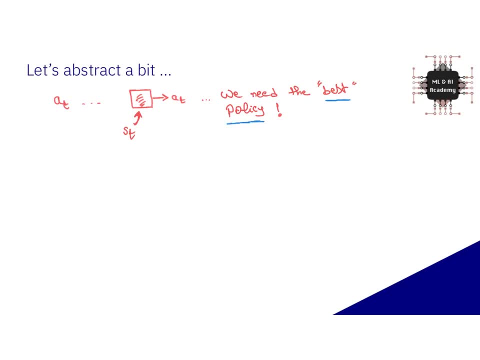 And what type of policy we're going to consider right. So now, the idea is that this policy itself- we can ask the question now, right, if this policy itself has to be deterministic, right or stochastic In general, you can actually use any of these forms, So you can have also a. 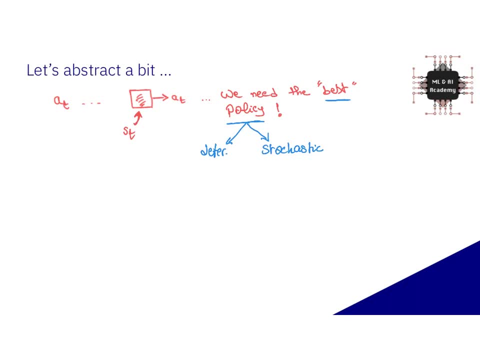 policy where you say, okay, let's draw a policy with the action and here we'll give you the same action- A, T. But here's the trick, or here's what's hard, Because we don't know the transition dynamics of our environment. we don't know that right. Remember P that dictates the transition. 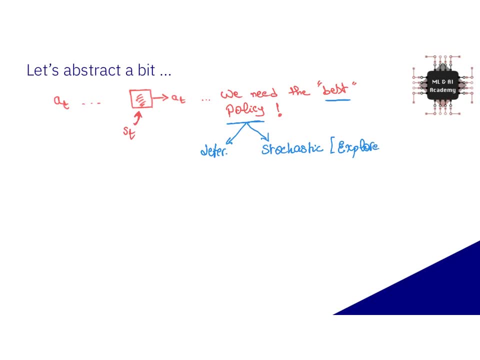 S T, A, T to S T plus one is not known to the agent. The agent is faced with a dilemma where it needs to explore, explore versus exploit. In other words, the agent can now use the current policy in order to always apply the. 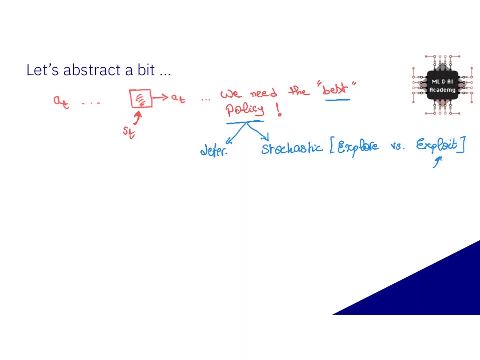 same action, sure, but that would not give it any additional information in that state st or the agent can pick to maybe take some form of a random action to get some new information about the environment, to learn something more useful about this xst. 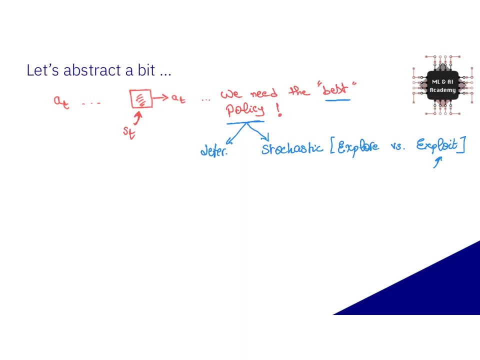 Because we have an unknown transition dynamics. what we're going to do is we're going to use a stochastic policy. So, as we used the old notation before, we're going to say now that the action at is conditioned on the state st and that is coming from some distribution pi, which is conditioned on st. 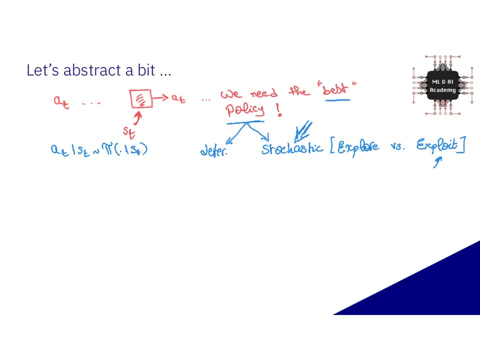 So again, this is a probability density which gives you a density over actions conditioned on this state. And now the goal of the agent is to find the best pi, such that it maximizes its performance. So again, because we have an unknown transition dynamics, now we require to have a stochastic. 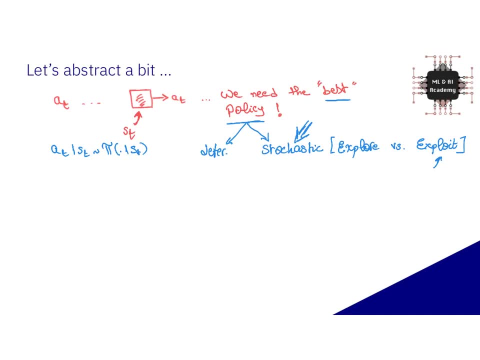 policy that allows this agent to explore new things around that state. So again, the goal of the agent is to find the best pi, such that it maximizes its performance. So again, because we have an unknown transition dynamics now, we require to have a stochastic. 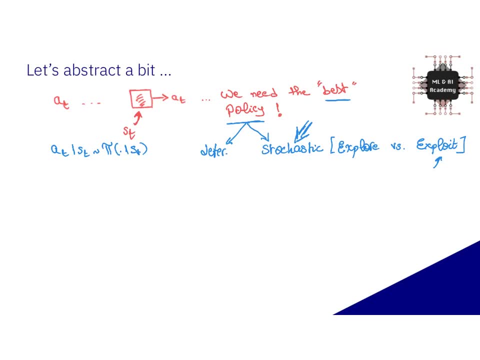 policy that allows this agent to explore new things around that state. In order to learn more and more, useful information is needed. So now, all good, We know what we mean by a state space, an action space, a transition model, a reward function, 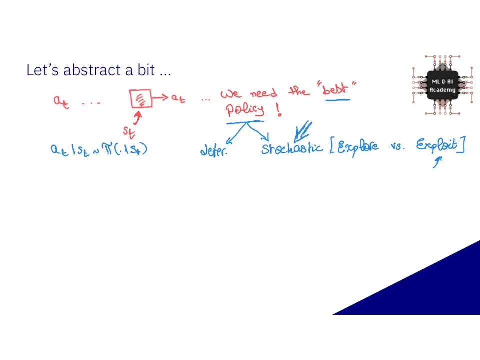 and now we understand what we mean by a policy. So now let's think a little bit about the dynamics of this reinforcement learning agent, right? So let's think about the dynamics of this repetition that we described before. So, as you recall, we had an action space, a transition model, a reward function, and now we have a stochastic policy. 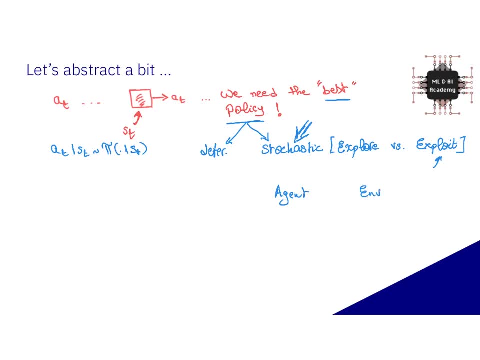 agent. we had an environment. the agent talks to the environment, the environment responds right and this process repeats over and over again. so we're gonna assume that it repeats- not forever. we're gonna just assume that it repeats for some horizon, big T, right. so I'm gonna execute this in a loop for some T steps. 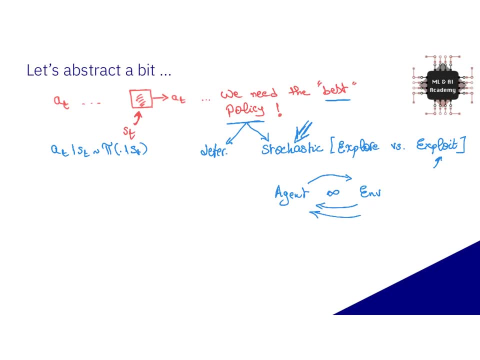 so now, as the agent interacts with this environment, what happens is that it will collect some form of a trajectory in that environment. so, for example, it will start at some state as zero which comes, maybe given to us, or some distribution or whatever. given this as zero, the agent is gonna use the policy pi that we have. 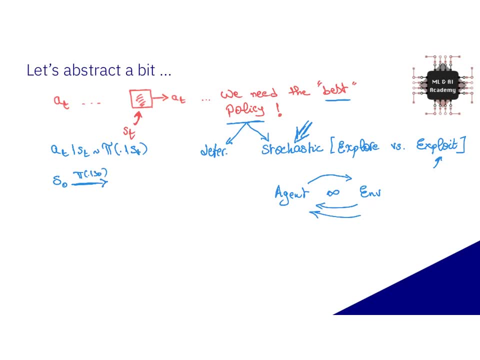 here in order to get an action- sorry, in order to get an action- a zero. so that's a zero. and then this will take me to some new state, as one, where that as one, as you recall, is coming from the transition model, as zero. a zero, right? so I start. 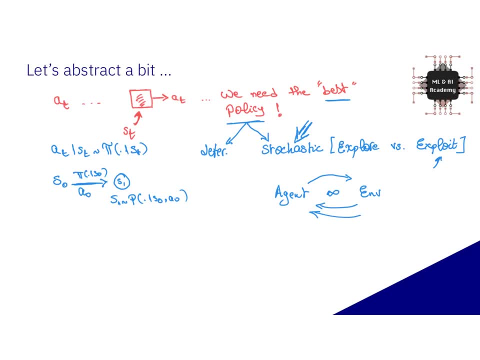 from some state as zero. the car is here. I apply an action according to my function rule of policy pi, so it says go forward. given that I am in a state as zero and I apply go forward, I will observe a new state, s1, which is maybe. 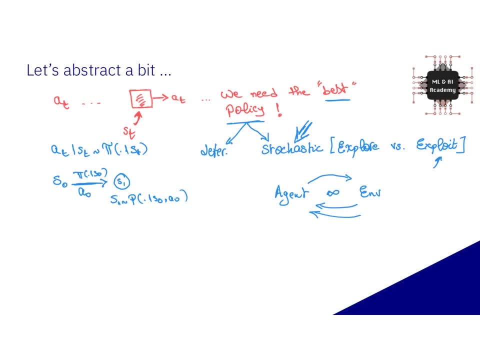 like ten meters or a mean couple of meters to the front, and that, as we said, comes from a stochastic transition. so that's why we say that s1 is sampled from p, conditioned on s0 and a0. given that we are at s1, this process then. 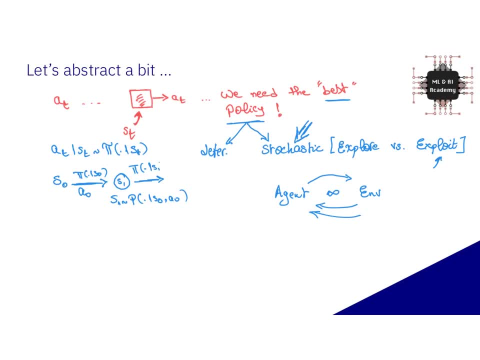 repeats. I query the policy pi for the first time and the argument is that S1 is not in an S1 state again, but giving it now s1 as my input state and then that will give me some action a1, then i will go to s2, right, so that give me s1, and so on up to reaching some horizon st. so this process repeats. 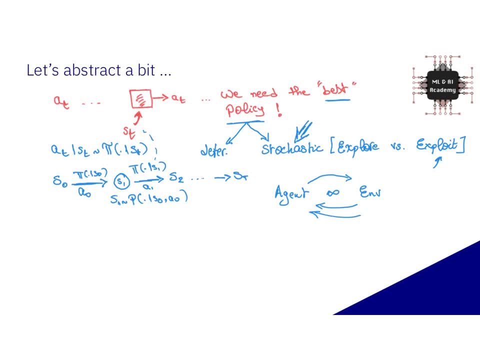 over and, over and over again by asking the policy what action i should take. the policy responds by an action. i put that action and that state to my stochastic transition model. it takes me to a no successor state and then this process repeats over and over again. we're gonna call s0, a0, s1, a1. 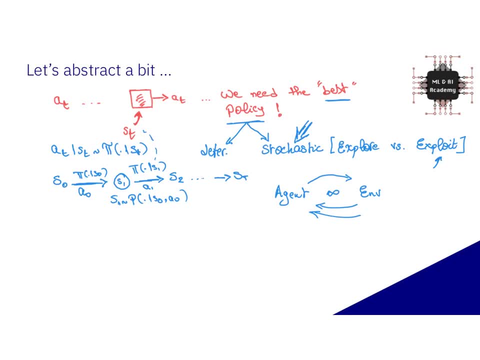 and so forth. right, we're gonna call that as a trajectory tau. so we're gonna define a trajectory tau and that trajectory tau is gonna simply be a collection of this: s0, a0, s1, a1, up to st right. so, as the agent interacted with the environment, the environment responded by some 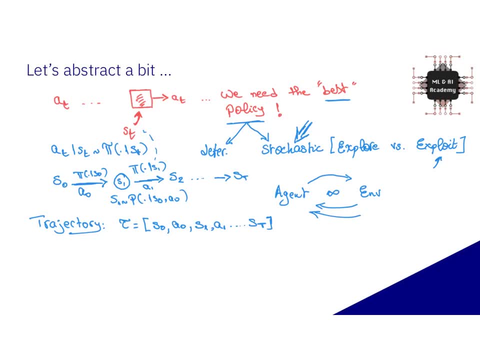 successor states, and also some rewards, which we will come to in a second. and then we're gonna collect all these s a, s a, s a and so forth and put them inside a trajectory which we will call tau. now, please notice that this trajectory itself is random, right? the thing is that because we have 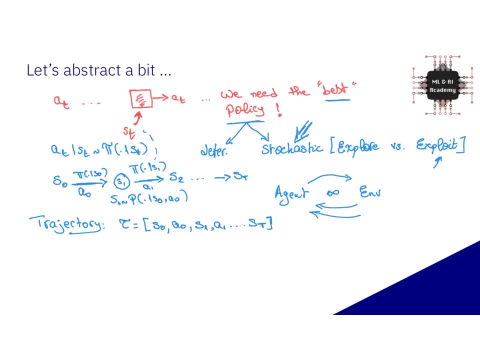 a random policy and a random transition. if i had started at zero again, i would have drifted off in a completely different trajectory, depending on the actions and transitions that i have sampled. so, in other words, this trajectory tau is not deterministic. it is a stochastic vector, depending on the actions you've taken and the transition models you've taken. 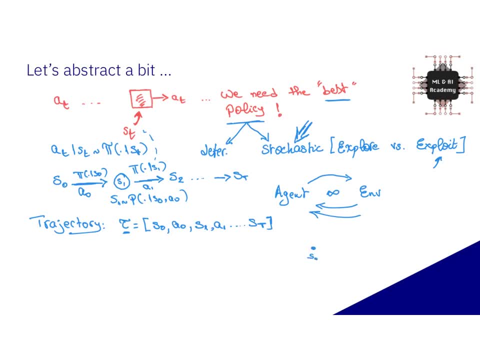 so, for example, if you had started from this s0 by, you know, applying some form of samples, you might have drifted to this trace, trajectory, or you might have drifted to this trajectory or trace, so you might have drifted to this trajectory or trace, and so forth, and that's why we cannot deal with this trajectory tau. 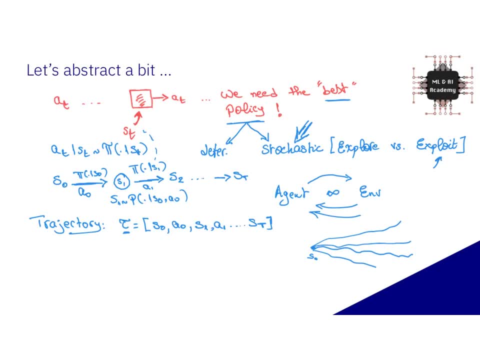 as a deterministic entity, but we need to deal with it as a stochastic entity for the reason that the transition model, as we agreed, is stochastic and the policy itself is a stochastic. so, with that in mind, we know that tau is a random variable. if it is a random variable, then i can define some form. 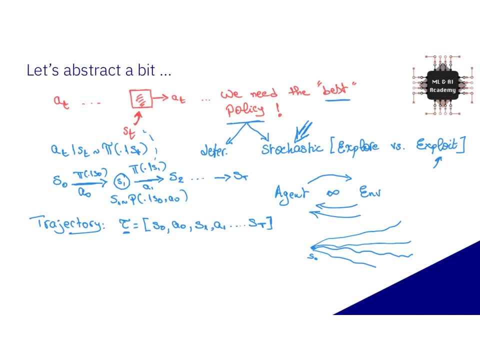 of a density over that trajectory, tau. so now i can ask the question of: what is p of tau? right, because we said that tau is a stochastic entity, so it is a stochastic vector. right, so now we can ask the question of: okay, if this is stochastic, because the transition is stochastic and the policy is stochastic. 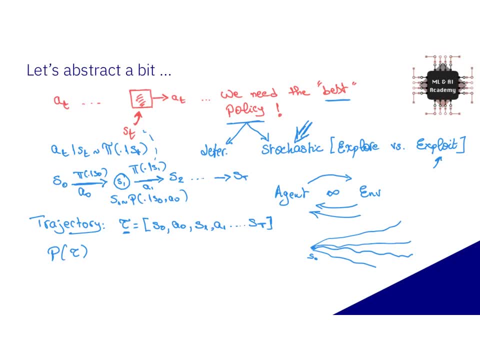 what is p of tau? what is the density over that stochastic entity, p of tau? what does p of tau mean? okay, so understand this. we know that p of tau is simply p of this. following joint distribution of s 0, a 0, s 1 a 1 up to s: t: really. 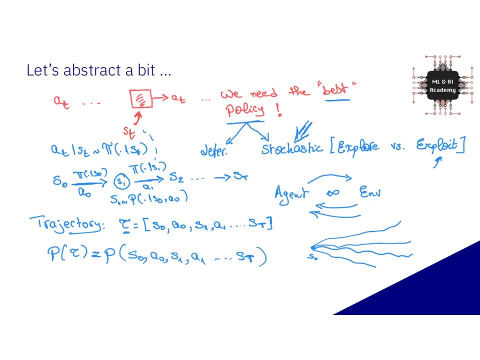 right. so what i mean by this is that the density over this random vector tau is nothing but the density over this intersection of random vectors: tau variables s0,, a0,, s1,, a1, and st- Each of which, by the way, is a random variable in its own right. 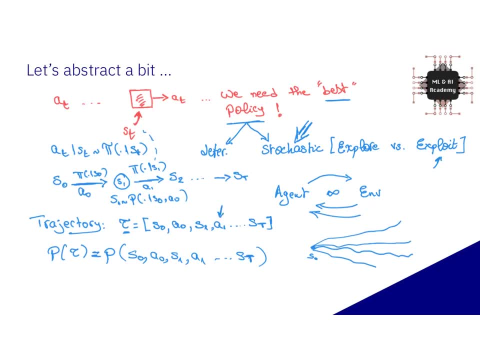 because a0 is coming from some, or at in general, is coming from some density. st is also coming from some density, right, because st is conditioned on st-1 and at-1.. And we also will assume that s0 is just coming from some initial distribution, Right? so now we have. 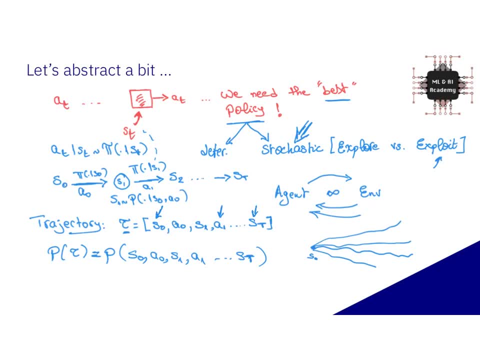 the question to answer and that is, what is p of tau really? Because we want to understand how would this density look like For this p of tau. All right, so now we can try to factorize somehow this joint density. 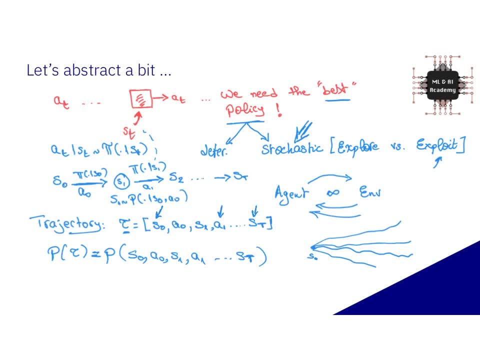 right, depending on some notion of density equations. right, And this notion is really very simple. The idea is, we can infer, In fact use, some form of bias rule in order to try to factorize this p of s0, a0, s1, a1,. 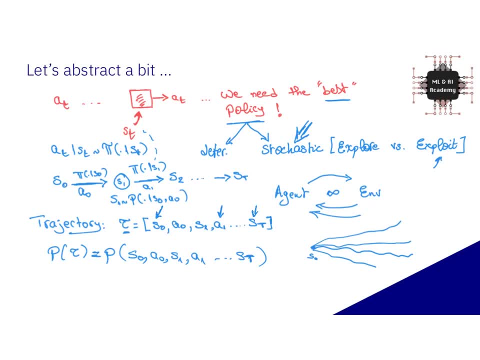 up to st. So the question is now. so here's the question we want to try to answer: How to factorize p of tau Right. so we want to understand how we're going to factorize this p of tau Right. so let's recap: We said that in RL we had a state space, an action space, a reward. 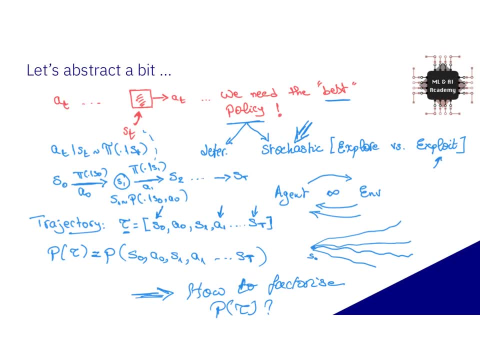 function: a stochastic transition model due to sensory noise, and then we introduced as well a stochastic policy type. Due to that, every time the agent interacts with the environment, what it will observe is some form of a trajectory tau, but that trajectory tau itself is random. 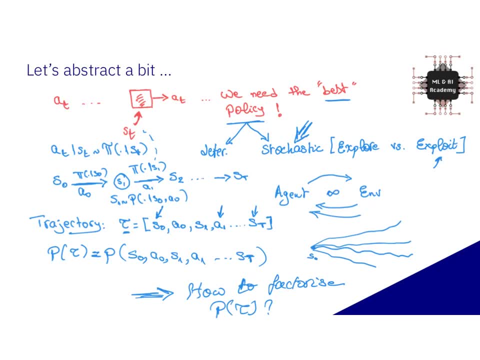 because the transition is random And the policy is random. Because it is random, now we can define some form of a density over that trajectory, tau, which is nothing but the density over this. joint random variables here as 0, a0, s1, a1, up to st. And the question we want to try to ask now is: how are we going? 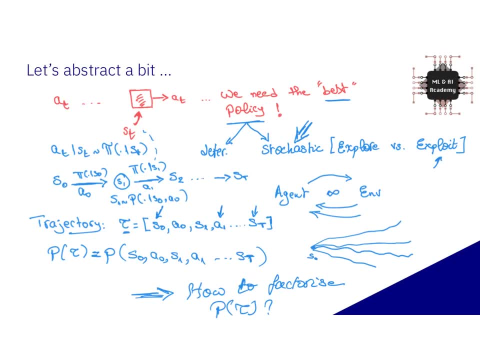 to factorize this p of t. Once we understand how we can factorize this p of t, then this problem of stochasticity becomes a little bit more complicated. So we're going to try to factorize this p of t Once we understand how we can factorize. this p of t, then this problem of stochasticity becomes a little bit more complicated, And we're going to try to factorize this p of t. then this problem of stochasticity becomes a little bit more complicated. So that's what we're going to do next. 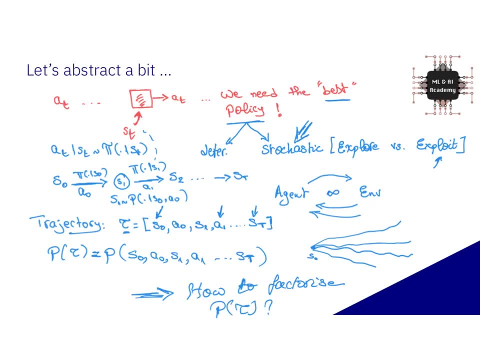 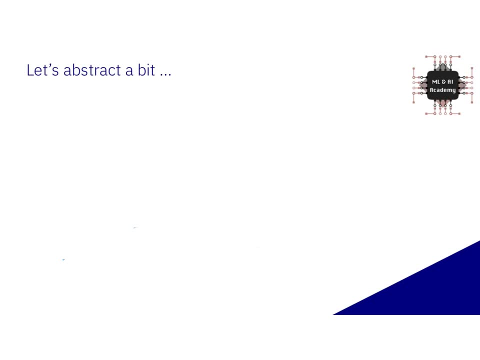 Alright, so, okay. so now we want to try to understand how are we going to try to factorize this p of tau, this density, over a trajectory that the agent exhibits, which is, as we said, P of S0,, A0, S1, up to S T. 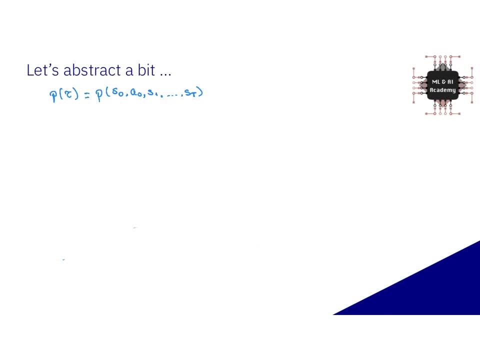 Okay. so in order to factorize this, we have to understand a very simple concept from probability, which is the chain rule. The chain rule says that if you have two random events- A and B- so say you have two random events, A and B, right. 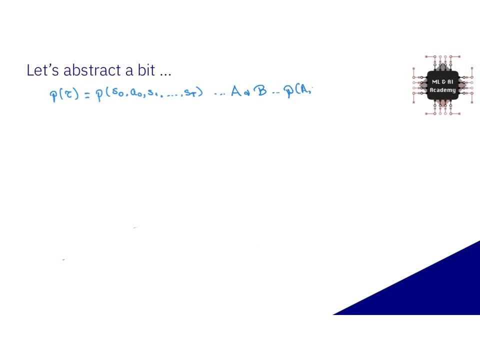 When you are interested in writing the joint of P of A and B right or intersection B, we can write this as P of B, given A times P of A. So the joint distribution over A and B can be written as. the joint distribution over A and B can be written as: 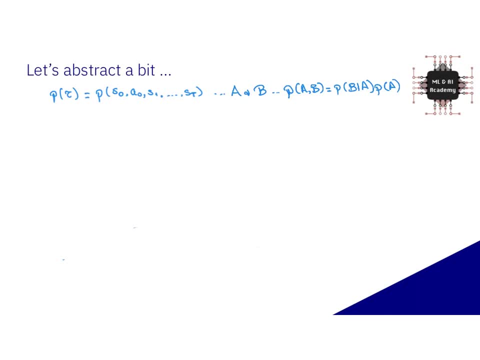 the joint distribution over A and B can be written as the product of the conditional distribution of B, given A times P of A. Now it's easy to prove this really. I mean, you can just use bias rule in order to prove this. 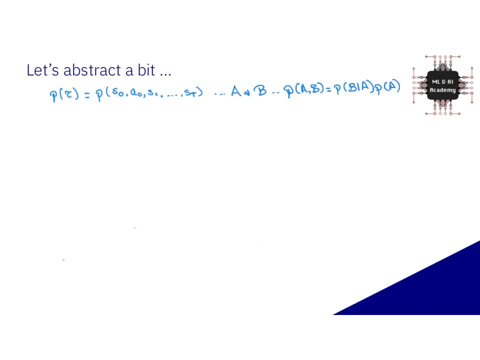 but we're just going to take it for granted, And the details of how you get this can be found in the other lecture of probabilities. But now we can in fact extend this to more than two events by saying that if we have a set of events- A1 up to An- 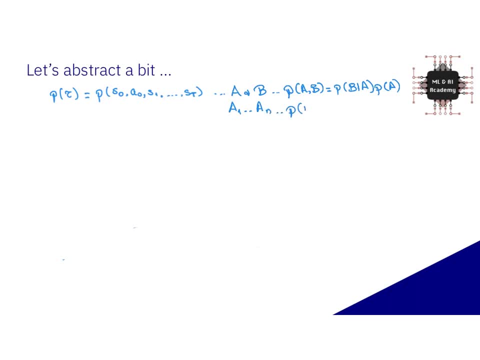 the joint of A1 up to An can be written as the conditional of An on An-1 up to A1, so condition the last on everything else times the joint of everything else, so An-1 up to A1.. So if you do like an induction proof, 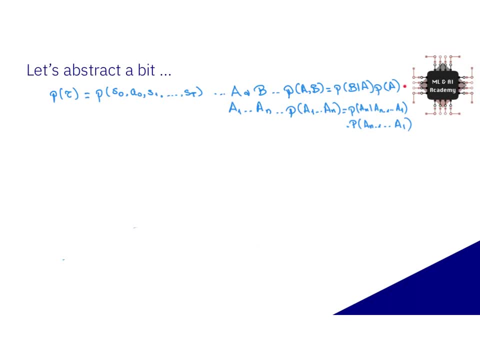 you can show that using this formula, you can in fact prove that the joint density over N events can be factorized as the density over the last event conditioned on everything else times the joint of everything else. Now, please notice that you can in fact 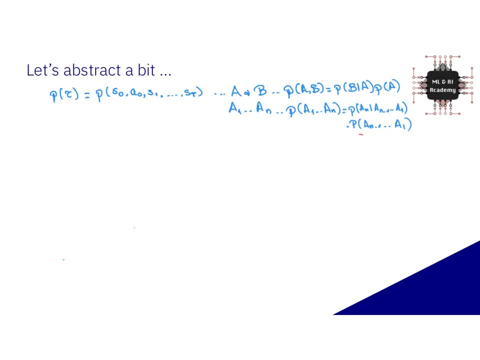 repeat this idea on this remainder here right, So we can still factorize this guy into P of the last, which is An-1 conditioned on An-2 up to A1, times the joint of An-2 up to A1,. 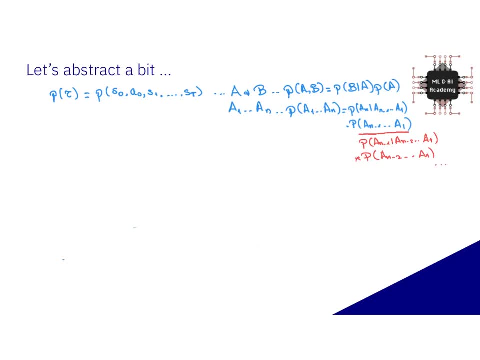 which is the remainder, And this process can repeat. You know, you can go back up to A1.. So now this is a, you know, very simple idea called the chain rule, Where we can condition the last on everything else, then multiply by the joint of everything else. 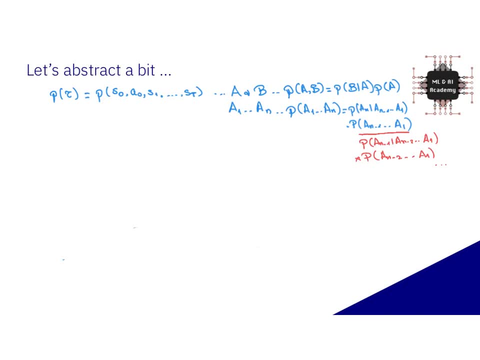 Let's take that idea and apply it to our problem here. So we're going to write: P of tau is equal to. So the last event for us, which is An here, is going to be S big T for us. So then we're going to say, okay, we're going to say P of S big T. 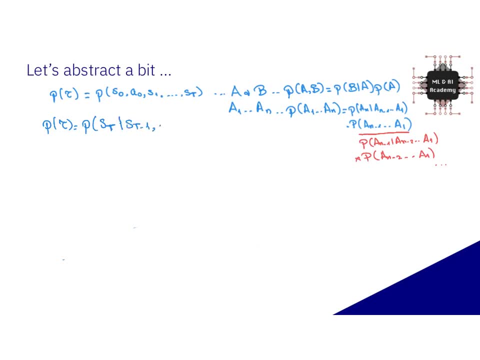 conditioned on everything else which is St minus 1, A T minus 1, dot, dot dot, up to S0 times the joint which is P of St minus 1, A T minus 1, up to S0.. 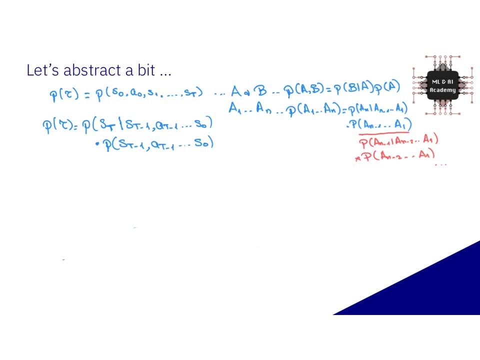 Good. So we just simply applied the chain rule from here, right From this equation to this equation. So we said we're going to have St conditioned on everything else, And then, Analogously, An conditioned on everything else, times the product or times the joint, times the joint of the remaining events. 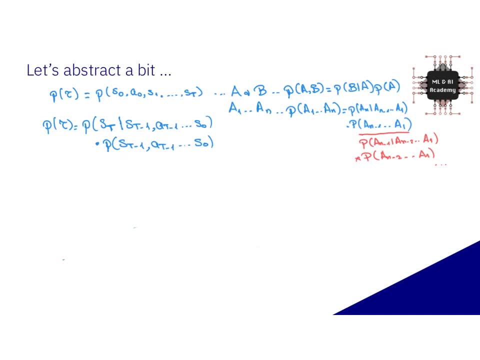 which is, in this case, is St minus 1, A, T minus 1, up to S0.. Analogously, here, the other remaining events are An minus 1, up to A1.. Now we're going to use an assumption embedded in the name of a Markov. 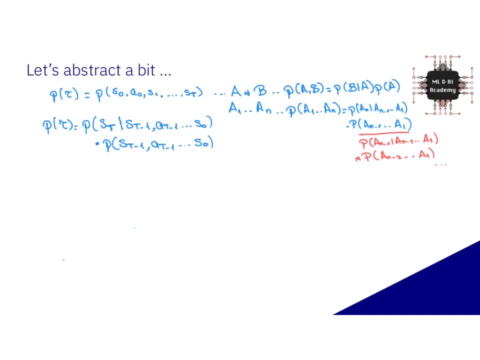 decision process. Markovian assumption says that the future only depends on the present, irrespective of the history. So what I really mean by that is that St itself, it only depends on the previous time step event, independent of the other history. This is what the Markovian assumption really says. 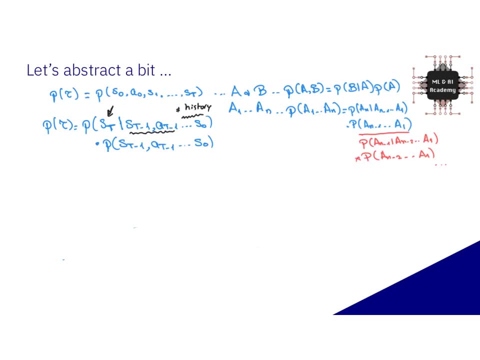 It's what it dictates. It says that the event now, which is St, is only dependent on the last step event, irrespective of the history, I don't care the path where you came from, but if you give me what is now, which is St minus 1,. 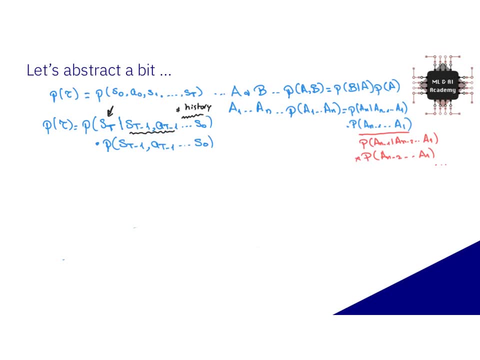 A, T minus 1, I can tell you what happens at S big T. So that's kind of the Markovian assumption. So, invoking that assumption, we can rewrite this. So from here to here we invoke the Markov assumption. 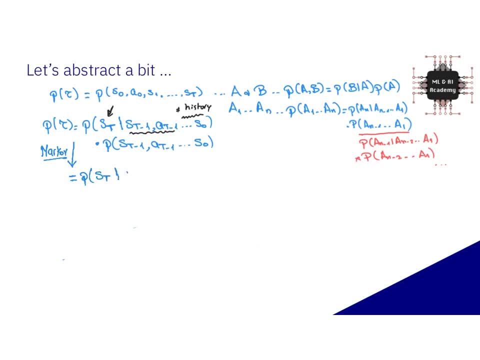 We can write this as now: P of St conditioned on St minus 1 and A T minus 1 times the P of the remainder, which is A T minus 1, St minus 1.. Up to S zero. So notice here I just flipped these St minus 1 and A T minus 1.. 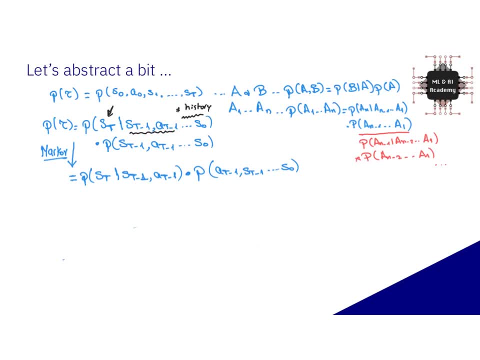 So it used to be St minus 1, A T minus 1.. I just made it A T minus 1, St minus 1, which is the same thing. So now it's interesting to realize that this here right, This thing here, is something we defined before, right. 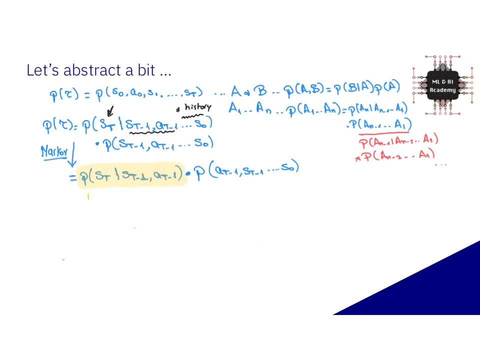 This is something we know. That is nothing but the transition mark. This is something we know, right. So it is this form of a model where you give it your St minus 1, your like previous state, previous action- right, And then it gives you your successor state. 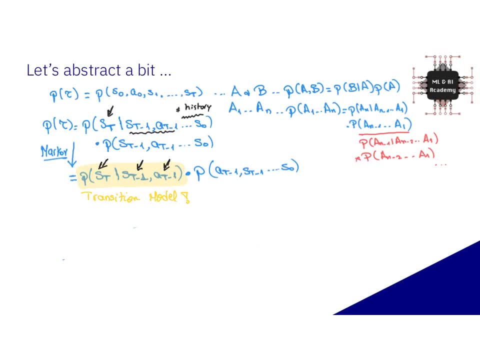 So that's interesting because it seems to me- I don't know, I don't know- But on the right track, because we're already observing components of the problem, of the MDP problem definition inside the trajectory, which is something that really should happen. 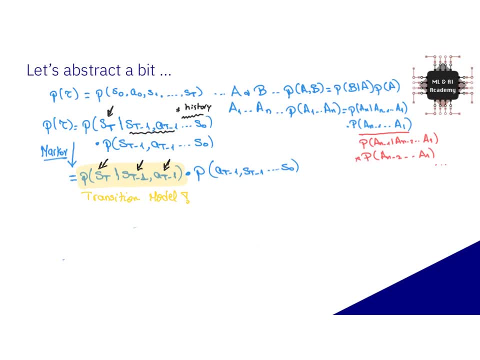 And now what we're going to do is simply, we're going to apply this idea of chain rule again, but for this entity here. So we're going to say that P A- T joint of A- T minus 1, St minus 1, up to S zero. 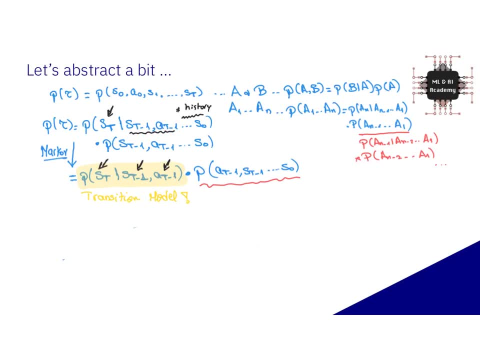 It's going to be again factorized into. so this can be again factorized into P of A, T minus 1, conditioned on St minus 1 up to S zero, right. So everything else times the joint of everything else, right. 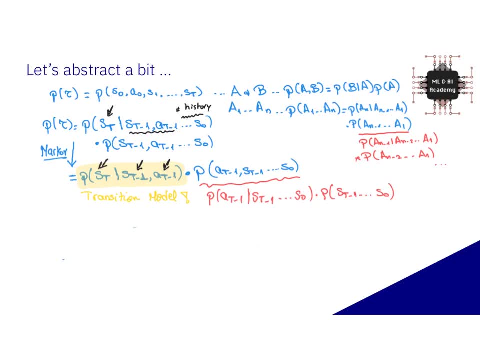 So all I did here is I applied the chain rule once again. So I said, okay, now I have A N minus 1, up to A 1,, which is A T minus 1 up to S zero, And that can be, using the chain rule, further decomposed. 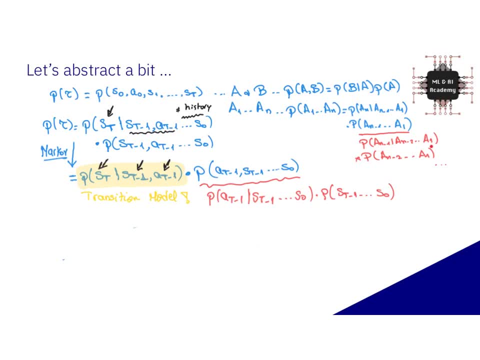 further factorized into A N minus 1 conditioned on A N minus 2 up to A 1, times the joint of the remaining A N minus 2, A N minus 1.. So I can factorize this into A T minus 1 conditioned on St minus 1 up to S zero. 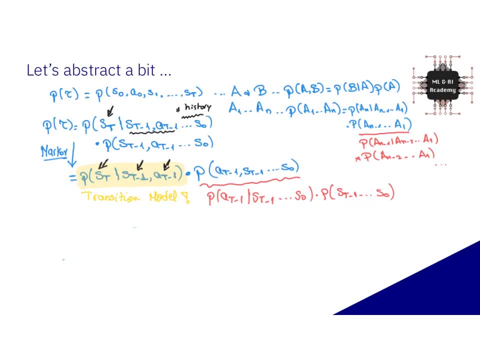 multiplied by the joint of the remainder. But now it's also interesting to realize that you know this itself, this guy here right, is nothing but our policy, Because it is some rule that, given your A, T minus 1, given, 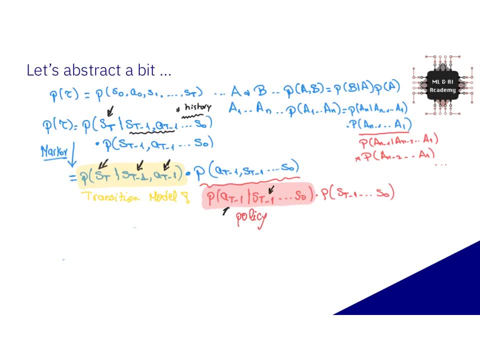 sorry, your S T minus 1, it should give you some A T minus 1.. Again, because of the assumption that we have a Markovian principle, which means that we can in fact get rid of all these history according to the definition of our policy. 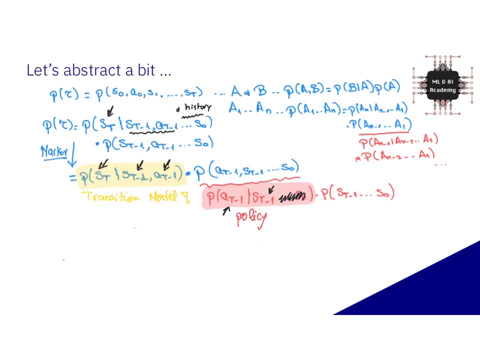 if you recall, and just say that this is P of A T minus 1 given S T minus 1.. So now that's interesting because we have the equation that looks like this: So you have S T given S T minus 1, A T minus 1,. 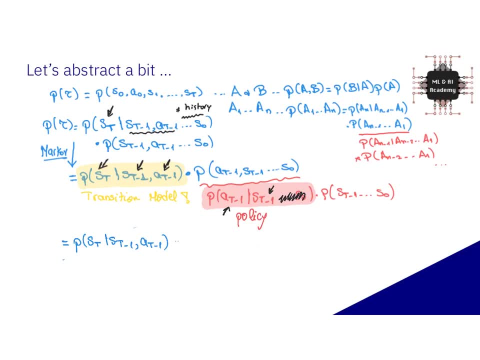 which is your transition model. Then you have the density of picking your action: A? T minus 1,, given that you were at your state, S? T minus 1,, which is your policy. And then you have this P S T minus 1 up to S zero. 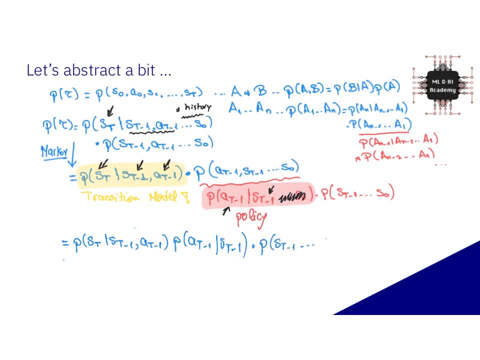 right. So then you have P of S T minus 1 up to S zero. Well now, by now you know, you know what's coming. So now you can just simply apply this chain rule over and over And over again until you go back to S zero. 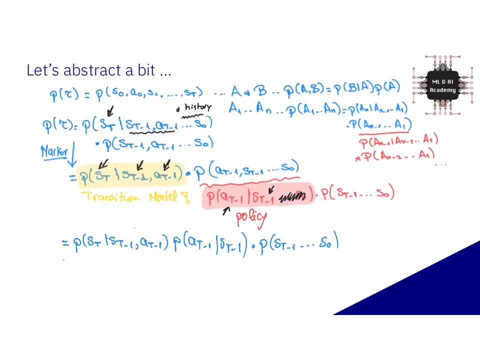 right. So you can say I have now S T minus 1 conditioned on S T minus 2, A T minus 2 times A T minus 2, given S T minus 2 times dot, dot, dot, dot, dot up to the first S zero. 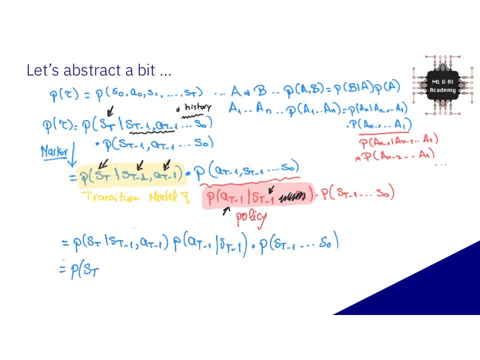 So what you can do now is you can write this as S T given S T minus 1 A T minus 1.. Then you have P S T minus 1, given S T minus 1 A T minus 1.. Then you have P of S T minus 1, given S T minus 2, A T minus 2 times P of A T minus 2, given given S T minus 2. dot, dot, dot, dot dot until you get back to P of S zero. 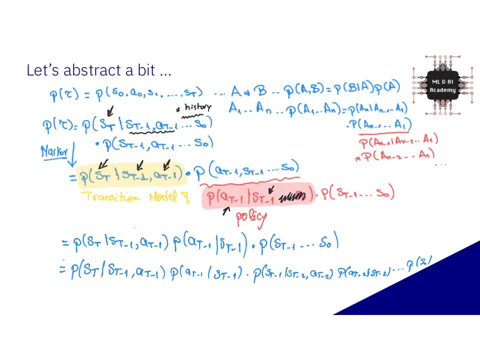 So just one word on P of S zero. What I introduced here is an initial state distribution. So I said that the initial state is sampled from some distribution. I mean that can be deterministic. but you know, I just assumed that there's some form of a given Gaussian. 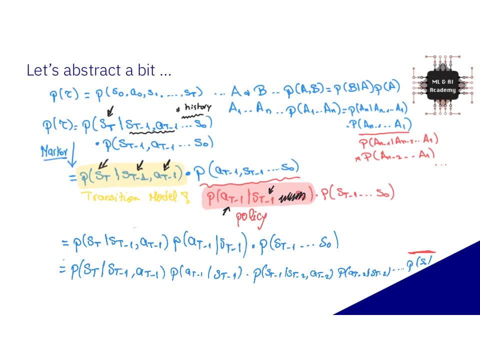 which gives me S zero. So in gym if you do n equal 3 set, that's, that's what this is supposed to be doing. But now I can just write this a little bit cleaner where I can say, OK, this is nothing but P of S, zero times the product over time. 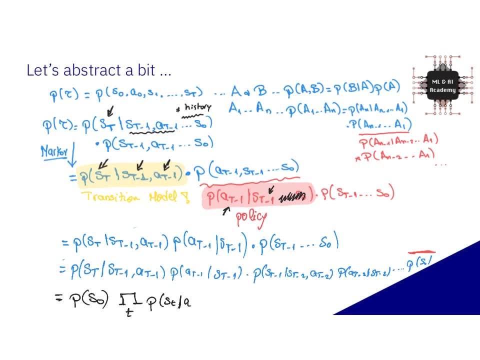 Of P of S T given. sorry, this should be right. So this should be S T plus 1 given S T and A T times the policy pi, or the P of A given S, which we just call pi, is just the notation we used. 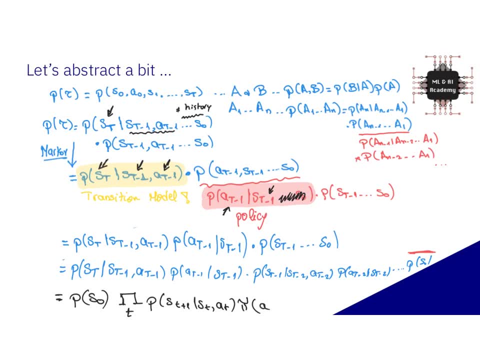 I mean, you can write this as P of actions. but yeah, A T given S? T. So now we? we were able to factorize the P of tau into this equation. So what I've done from here to here is I've simply just rewritten this. 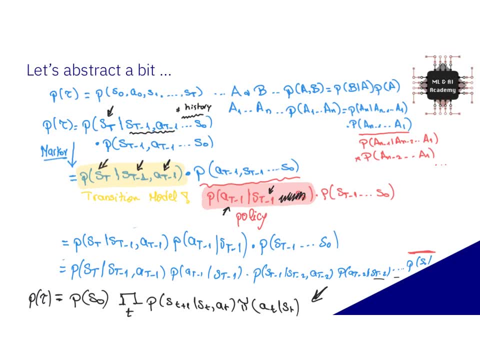 in a more concise form, right? So I took P of S zero right. I put it there because it's not conditioned on anything else And, as you see here we always have this product of S? T, given: S T minus 1, A T minus 1. 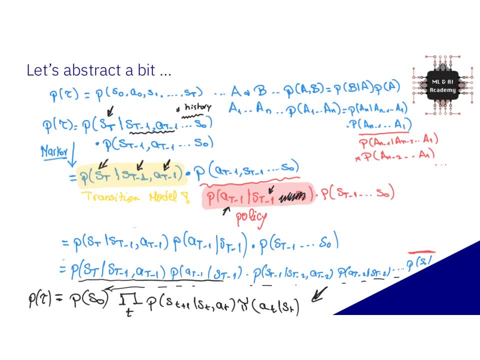 and A T minus 1, given S T minus 1.. So then I just put them there And then I had a product over time which yields back this equation. So now we were able to factorize the density over the trajectory tau into this form. 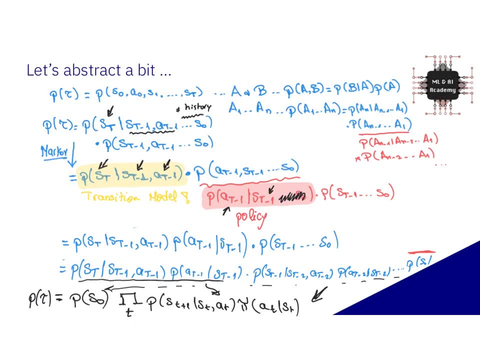 And now it's interesting to understand this form intuitively, because this is a very intuitive equation. So what this is saying is that imagine you have like this space here, right? So like the space of states, cross actions, cross time Or no, without cross time, because that will be a point. 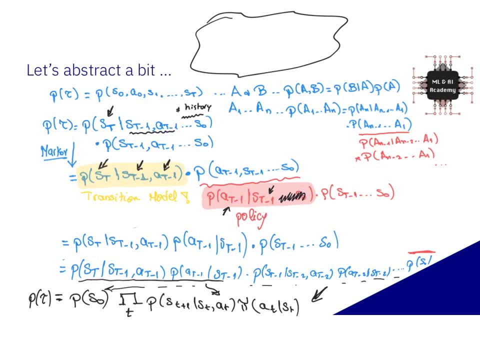 but just space of states, cross sections. What this guy is saying is that the first thing the agent will do is it will start from some S zero coming from P of S zero, Then it will take an action, A zero right, And then that will take me to S one. 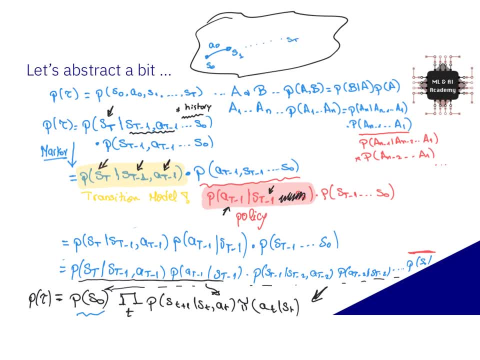 And so on up to S T. The density of this trajectory is simply the density of starting at S zero, picking the action on that state, then transitioning according to your transition model. So the way the density of the trajectory works is really intuitive. 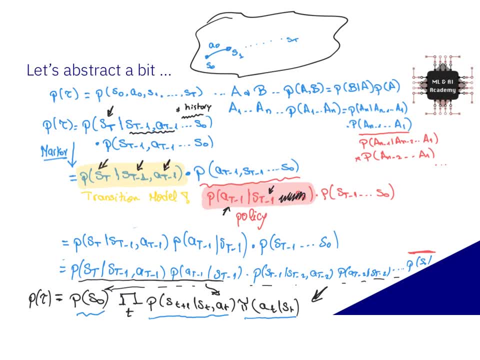 because you start at some place, you pick an action according to some distribution that takes you to another place And that's what's reflected by this product. So you start at some place, then you pick the action According to your policy that it takes you to your successor state. 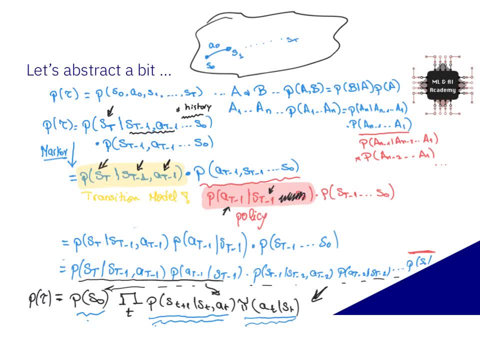 S, T plus one given S T and A T Dependent on this product over time itself. So now that we have understood how to factorize the trajectory in a reinforcement learning problem, Next what we're going to do is we're going to finalize this lecture by defining the 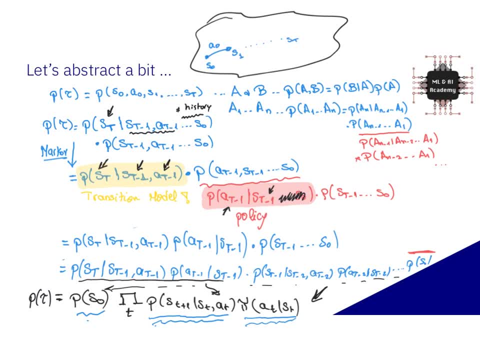 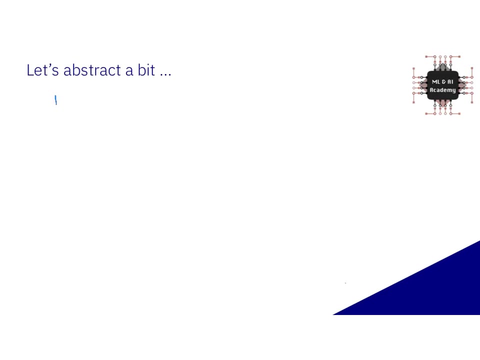 optimization problem We would need in reinforcement learning. So what is the agent going to be looking for, Right? So we so far have shown that P of tau right can be written as P of S zero times this product over time of P of S T plus one. 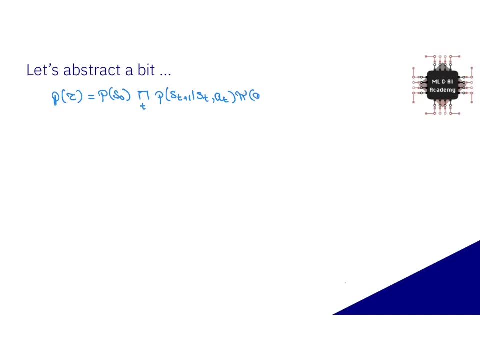 Given S T A T Times the policy of applying A T in S? T. So now okay. so now we understand that, and then we need to think of some notion of measure that will allow the agent to learn a good action selection rule pie. 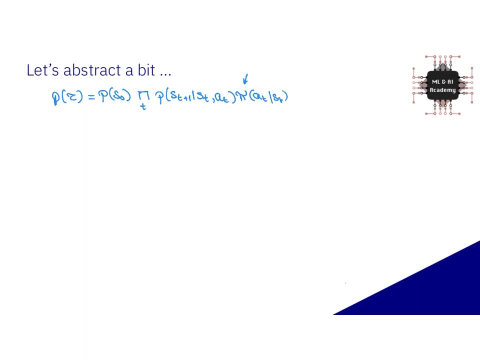 Right. So remember, in the previous slide, we said that our goal is to find the best policy, and now we need to understand what do we mean by best. Okay, in order to understand that, we're going to now think a little bit more about the. 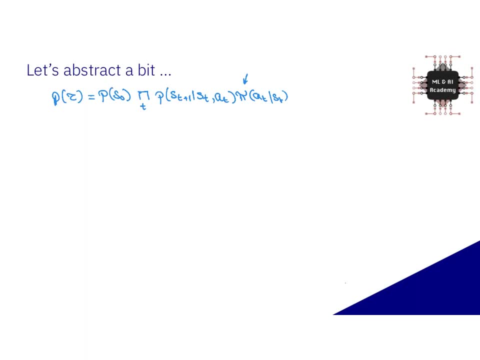 reward that we get over a trajectory, tau. So remember that you know we have this interaction of the agent And the environment and we said that the agent takes an action, The environment gives me a state and a reward. So so far we have handled these two components. 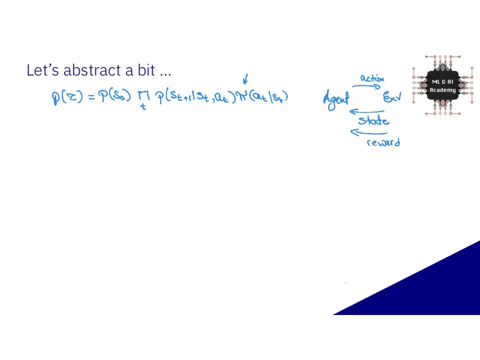 the action of the state, but we didn't talk about the reward yet. Well, what we're going to say is that for every trajectory tau, we have a reward, which we're going to call our total of tau. So the idea is that for every transition that you would get state and action. 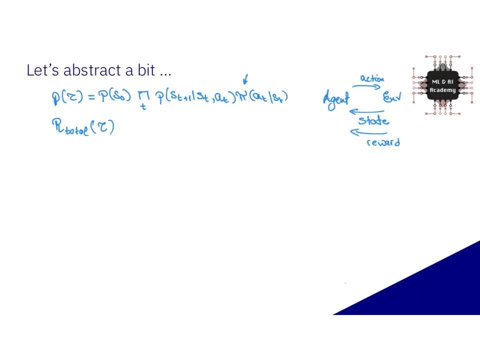 you will get a reward value corresponding to that state and action. So, as you recall, we defined the reward function R to be from S cross A to real numbers, which means that at every state, action pair STAT, this reward right is going to get for us a specific value. 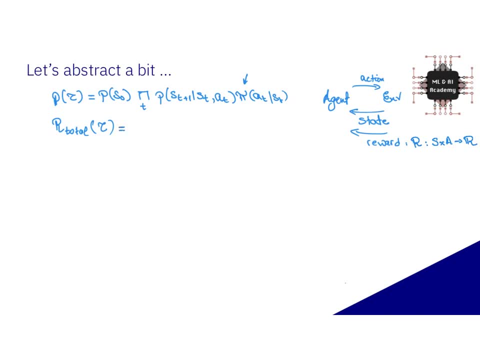 So, therefore, what we're going to do now is we're going to say that we have a function of these transitions in the trajectory S, A, S, A, S A. We're going to sum them up and that reward of STAT- It's over some overtime- is going to be the total reward of that trajectory. 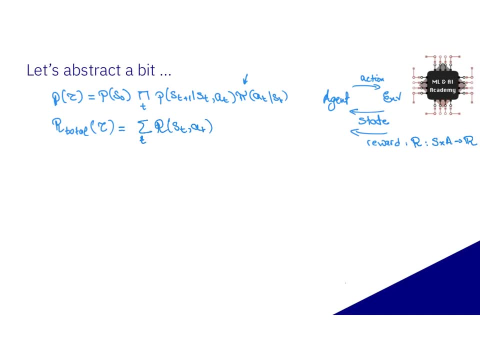 So how good a trajectory is that the agent has taken is simply going to be the sum of the instantaneous rewards That the agent has achieved throughout this interactions with the environment. So, for instance, let's say: this is the goal right And this is the starting state. 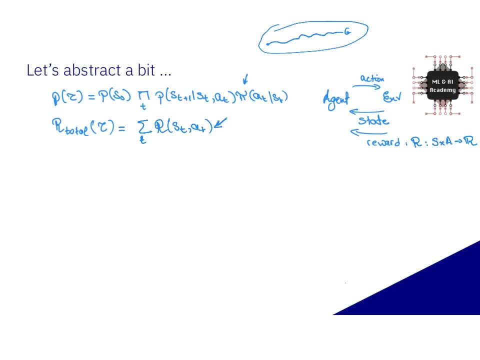 This reward. this trajectory will have a higher reward than a trajectory that looks like this, for example. Why? Because, well, it has achieved the goal. and the way we call did this reward function is that it gives me higher numbers If I achieve the goal. 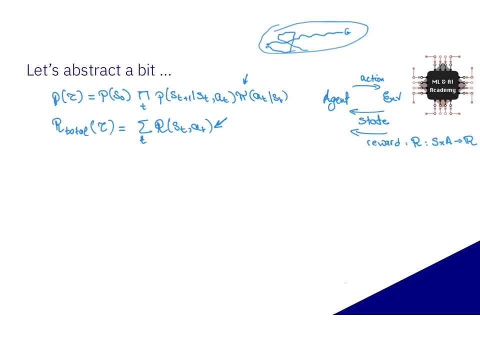 Now, by no means this reward is dense in this. reward can actually be very sparse, And that's what makes the reinforcement learning problem really difficult, If the reward itself is extremely sparse. So if the reward function was not like some form of a distance of approaching a 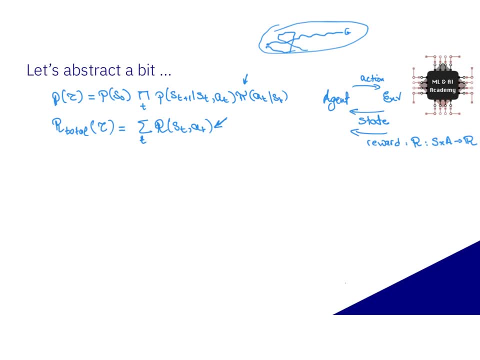 certain goal but was more like zero and one where zero if you didn't reach the goal and one if you reach the goal, then you can see that the numbers you would get for different trajectories that have not achieved The goal. 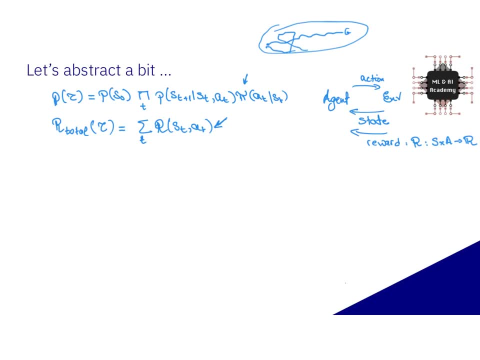 Are going to be zeros, which means that that's not much information And that's why it's hard to learn and reinforcement learning. but all these details we will come to later, But for now we're just trying to do the problem definition. 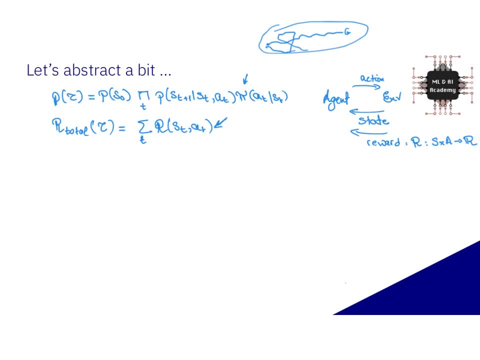 So please understand that now the report of the trajectory is nothing but the sum of instantaneous rewards that you get along that trajectory. And please, please remember right that the trajectory itself is random vector, because that's why we had to define a density for that trajectory. 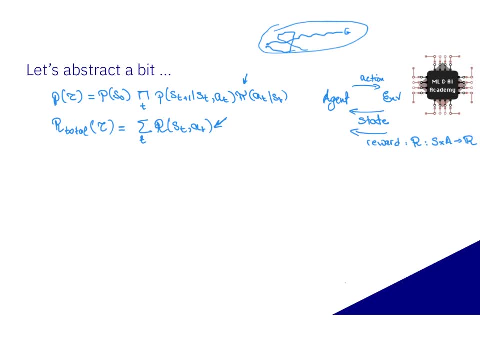 P of top. Consequently, Now, if we are to measure the performance across style, we need to handle that in some sort of a stochastic manner. We cannot say, just give me our total towel to be maximized for one towel, Either you have to do it over all towels. 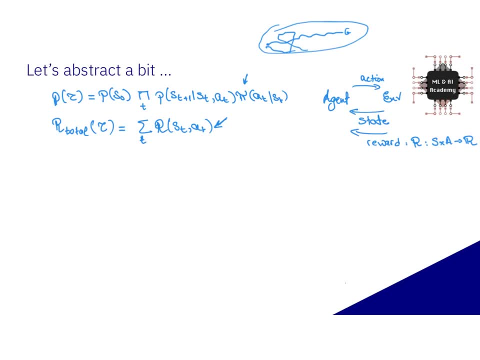 So for every towel you want that to be maximized. but that's a very, very hard problem definition, because you will have infinite number of possibilities. Or you can say on average, I want a policy that gives me a big R total. 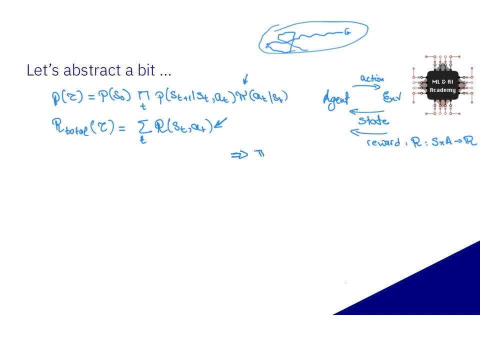 So what I want to say is that I want a policy pie. I want a policy pie that gives maximum R total On average Over trajectories Top. So this is an intuitive explanation, right? So we want to have a policy pie that gives me the maximum reward on average over trajectory style. 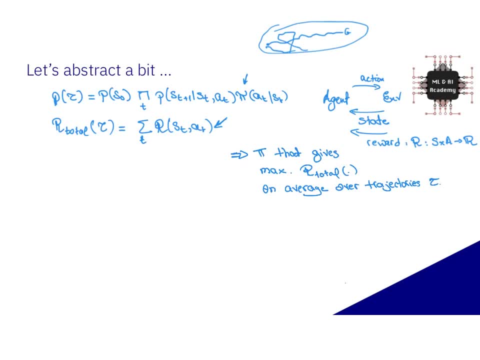 So now, what does on average mean right? So what does on average mean Well, mathematically, on average means expectation. So you want to have a policy, So we want a policy. We want A policy That does well. 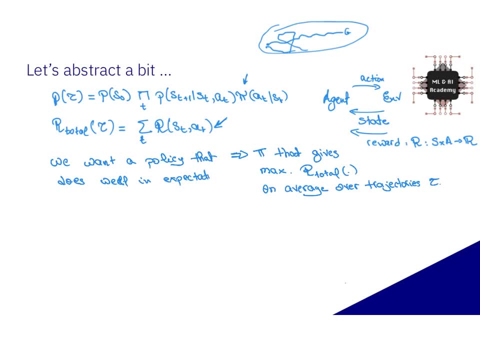 In expectation Over trajectories tell. So, in other words, we want to maximize with respect to, To the policy pie, because we want a policy that does well, which means it gets the maximum R total on average, which is an expectation Of the reward are total. 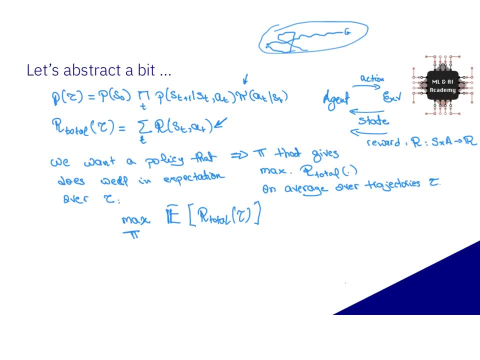 Over town. So now what we want is we want to get a maximum Reward total on average and we want to Find that policy pie that will give me that best performing reward total of these trajectories. Now, if you remember the definition of expectation, 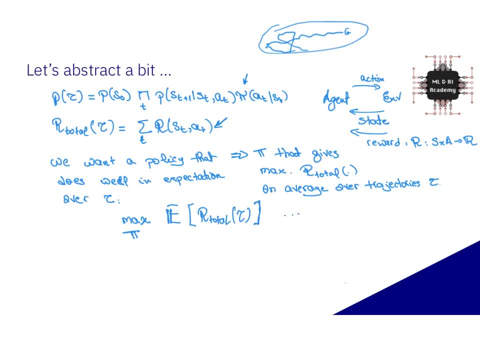 right. So if you had some random variable X and now you try to do E of a function of X, That is The integral right. If X is continuous of P of X, F of X, DX, right. So if you want to try to find the expectation of some function of a random variable X, 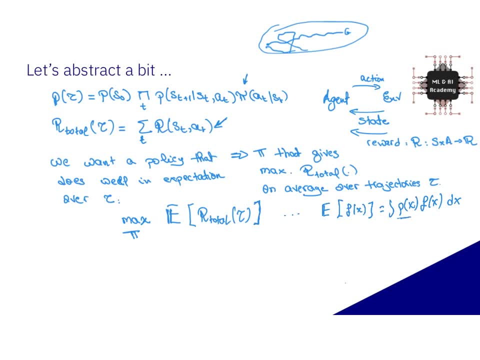 that is nothing but the integral over the distribution over or the density of P of X times F of X DX. So if it was discrete you would have a summation P of X, F of X DX in continuous. It's just the integral P of X of X- DX. 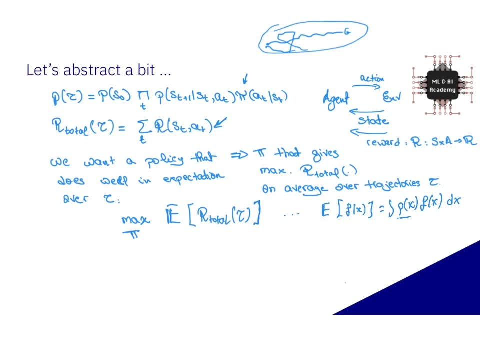 So when I write X is sampled from P of X, So E of X sampled from P of X, of F of X, I mean nothing but this definition. So I mean that this is E over F of X, where X is a random variable coming from. P of X is nothing but the integral of P of X, of X DX. 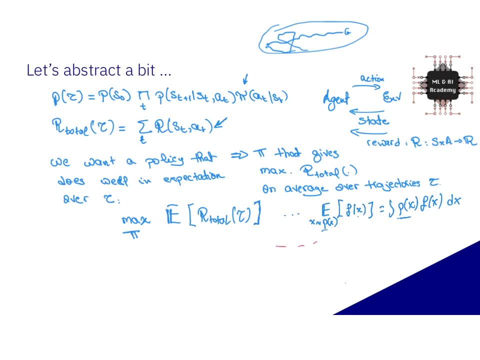 So, to take this notation To our scenario here, Tau is our random vector, right. And now what we're going to say is we're going to say that we want to maximize E over Tau Because it's our random vector, but Tau is sampled from what? 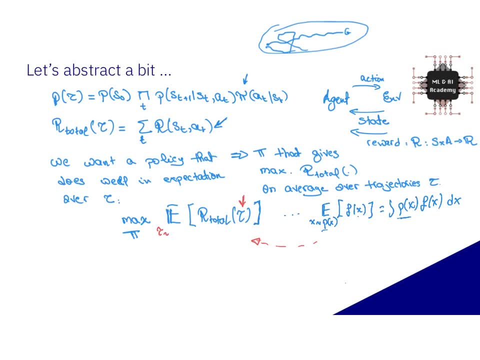 Well, it's sampled from the density over trajectories which we just derived. So that is P of Tau, R of Tau, And of course some people would like to put P? pi here, because that depends on pi. That's what the agent can control. 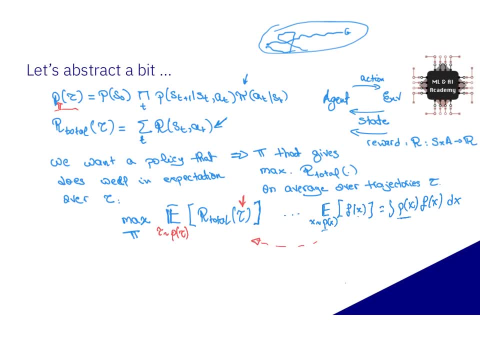 Of course it's pi and transition, but transition we cannot control. So that's why we just put P of pi, And I can therefore write this as max expectation over trajectory sampled from P, pi of Tau, of R, total. So what this equation is trying to say. 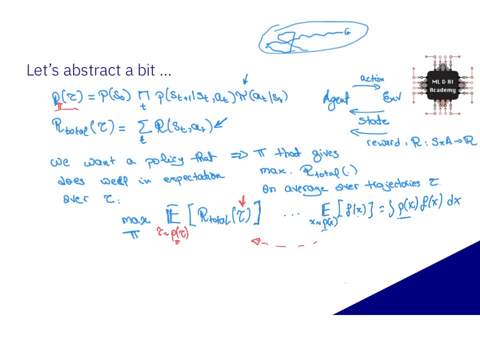 give me the best policy that, on average over trajectories, tries to maximize the total reward of these trajectories. And that is the definition of a reinforcement learning problem And that is: you want to try to maximize the total reward on average over trajectories, As we said. 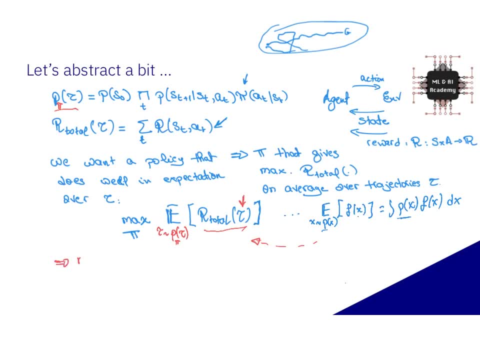 please notice the definition here. So, as we said, like just to be clear, max over pi, E over Tau, sample from P pi is the same as saying that's the integral over P pi of Tau, R, total of Tau, d Tau. So there's a density for the trajectory and that density is multiplied by the function d Tau. 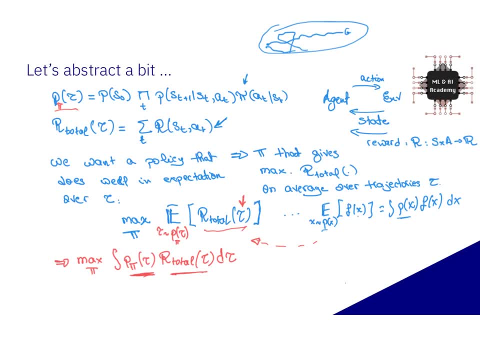 So in other words, integral of P of X. F of X was the expectation over X, sample from P of X of F of X. Similarly, here we can say: E of Tau, sample from P pi Tau of R total, is nothing but the integral over P pi Tau, R total, V Tau. 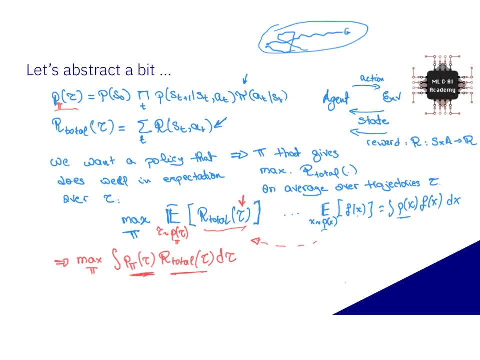 So that is the definition of the reinforcement learning problem And in the coming lectures we're going to dig deeper into how we solve this problem. And the current literature in RL is really trying to handle this problem, but in different ways. So we're going to talk about some approaches to solve this problem. 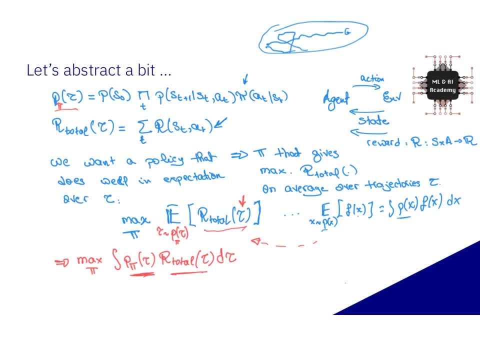 And of course, the later lectures will be a little bit more practical. We will where we will implement some of these solutions in OpenAI Gym. But this lecture set forward the problem definition of reinforcement learning And I hope it's clear enough to understand. 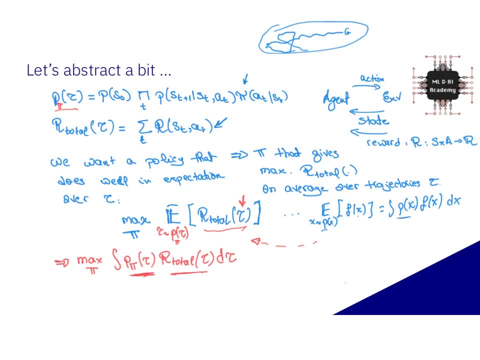 why this method is cool, because it covers a broad range of applications and how we achieve this problem definition, starting from the definition of the MDP to the definition of the stochastic policy and the stochastic transitions, to understanding the density of P, pi, of Tau, to getting our final problem definition, 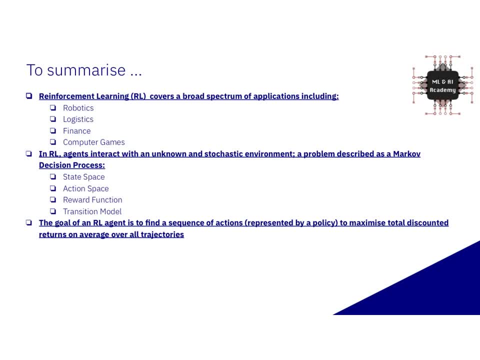 Right. So, to summarize, we know that now reinforcement learning covers a broad spectrum of applications, such as robotics, logistics, computer games, finance and so on. We know that agents interact with stochastic environments and the problem is described as an MDP or a markup decision process. 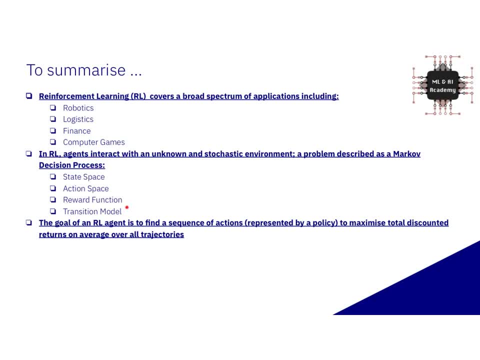 And that is represented by a state space action, space reward function transition model. The transition model itself is a stochastic. The action space dictates the type of policy you will use, which is also stochastic, And the goal of an RLA agent is to find the sequence of actions. 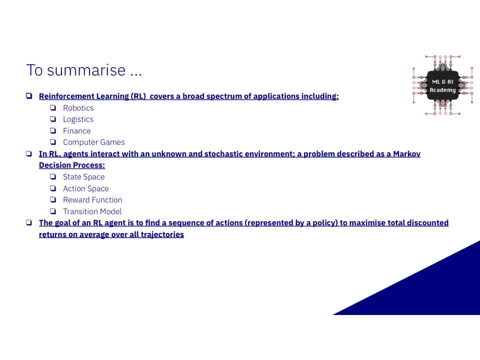 which is represented by the policy, to maximize the total return on average over all trajectories. And mathematically that meant to us that we want to maximize, over the policies, the expectation, over the trajectory sampled from the policy, from the density which depends on the policy, of our total 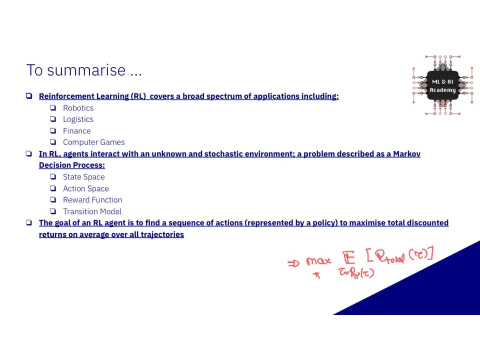 of time. So this is our goal And that's what we want to try to talk about in the next lecture: How are we going to be able to solve this type of problem? And we're going to categorize different reinforcement learning solutions. 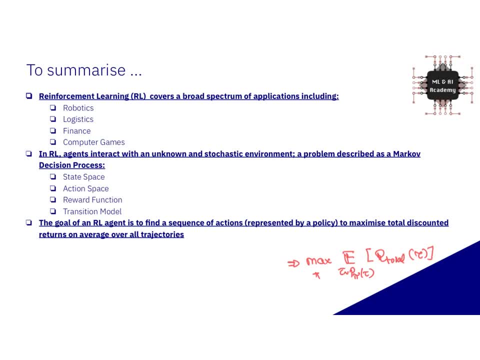 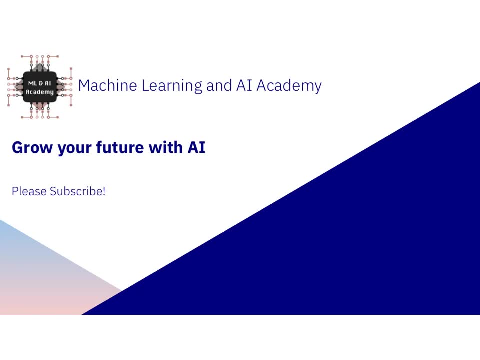 So maybe until then, it's worth thinking How would you approach solving this problem, Right? So thank you for following us in this lecture from the Machine Learning and AI Academy, where we hope that you will have the ability to grow your future with artificial intelligence. 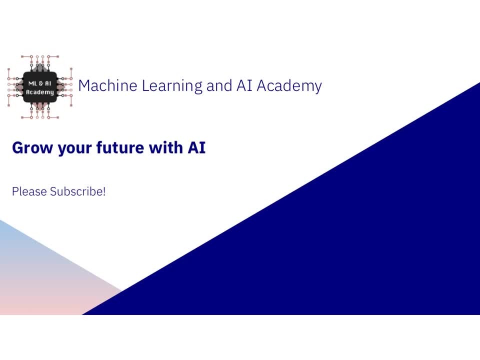 So we're now just discussing reinforcement learning, specifically deep RL, and we're going to detail some of the applications as well as the implementations of that. But in the future we are also planning to include different topics of machine learning algorithms, such as deep learning.